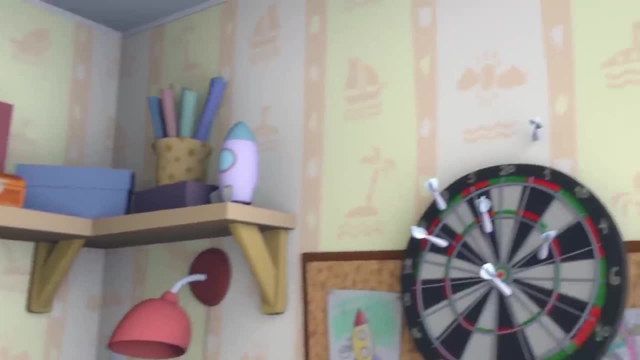 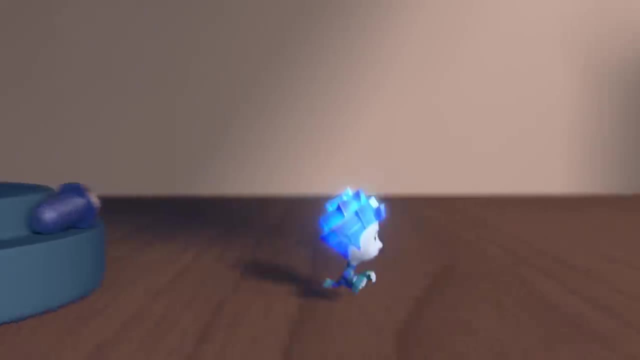 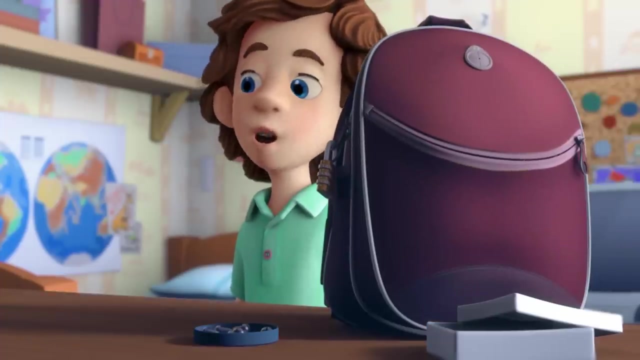 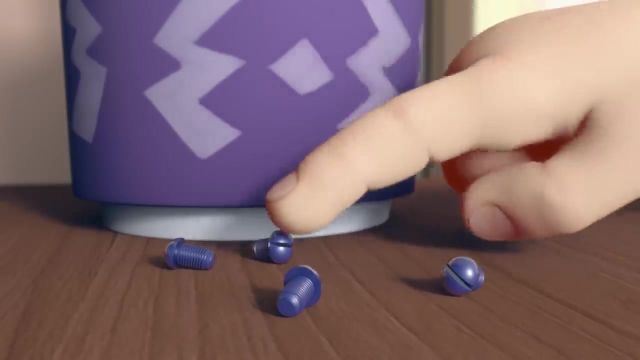 Subtitles by: Subtitles by the Amaraorg community. Ah, He's home. Nolik, are you here? Stop your hiding, I'll still find you. Nolik, is that you? Hey, come on, that's not fair. 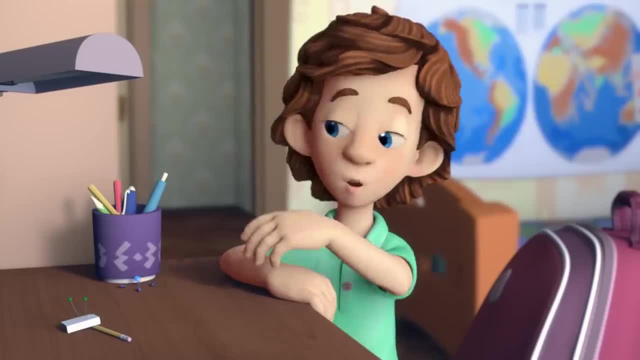 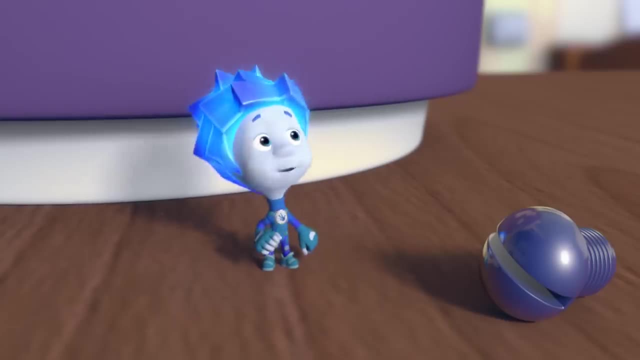 You saw, Let me go again. I don't want to. You want me to play hide and seek. when I got a brand new game to play with, Where is it? I don't see it anywhere in the room. I took it to school with me. 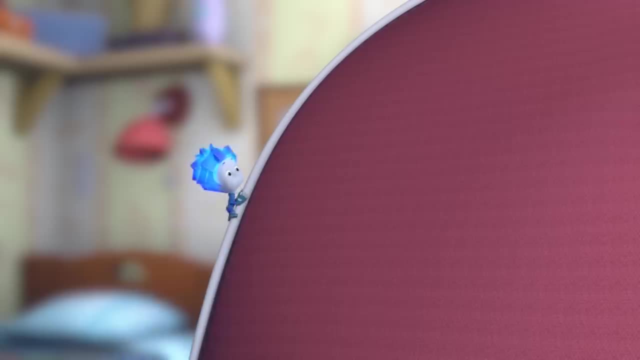 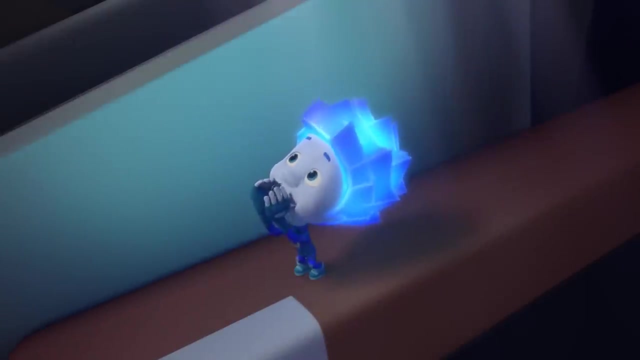 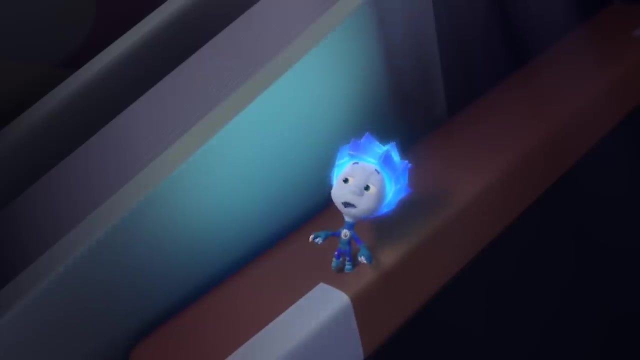 For what reason? To show it off. Wow, Awesome game. Tom Thomas, Can I play your game? Uh-uh, Because I'm not done playing with it yet. Now just try asking me to do some favor for you. Hmm, wait, was it a three or a four? 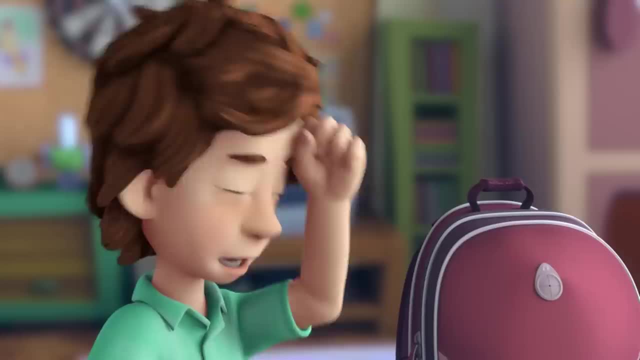 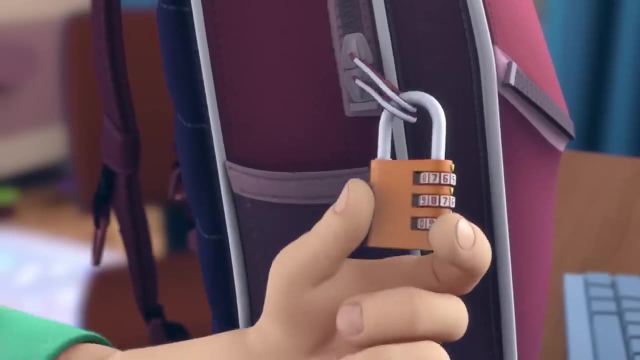 Hmm, it could have been five. I forgot. What about? I forgot the combination And now I can't even do my homework. Everything I need to finish is inside of there. I'm not climbing in to find out your homework. Don't even ask me. 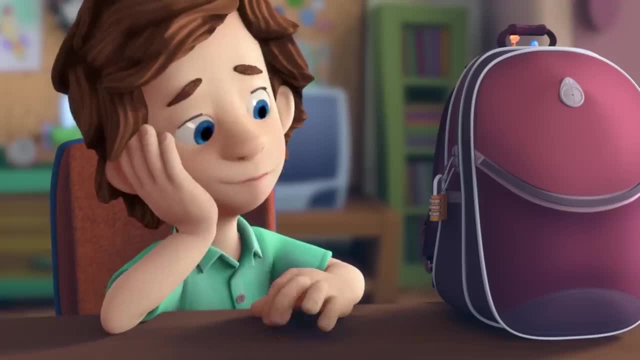 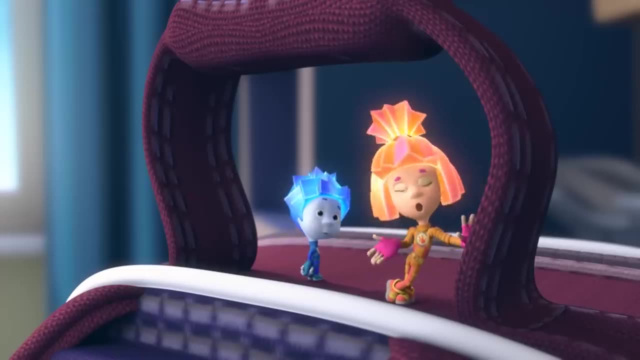 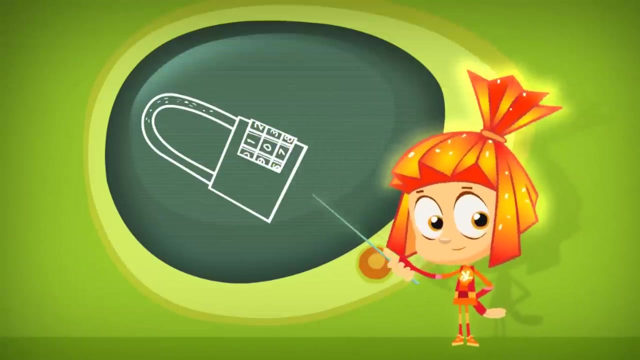 Tom Thomas, why do you look so upset? Ah, The code For the lock. I don't remember it, Don't you worry. Ha, We'll open it. I know all about a code lock. A simple code lock is built with a few disks that have numbers on them. 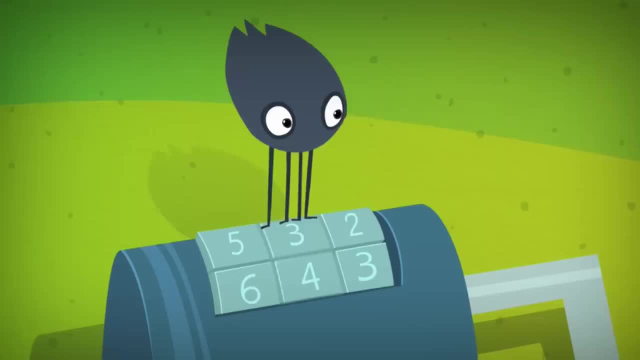 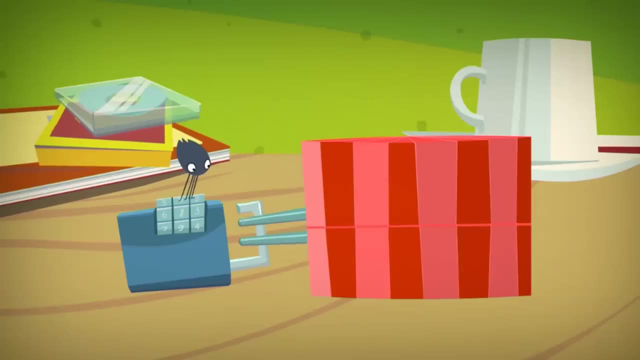 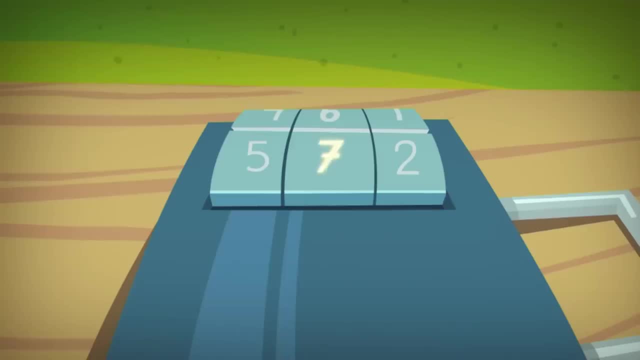 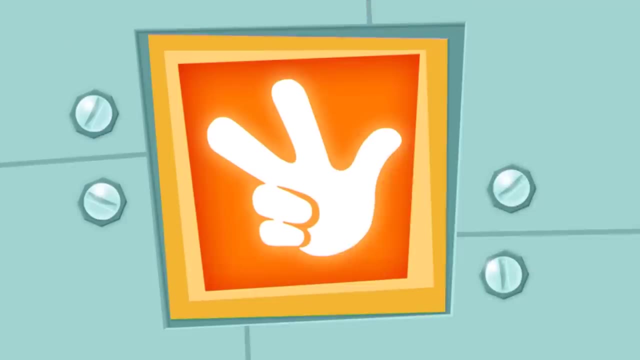 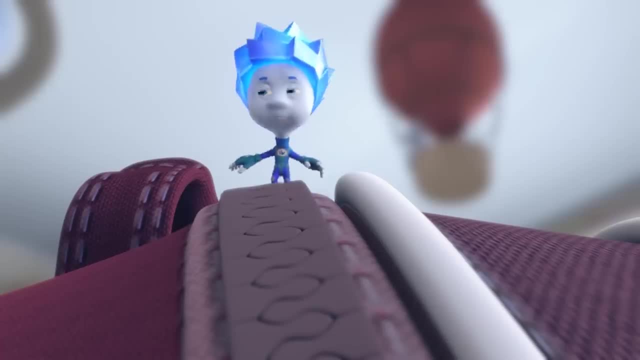 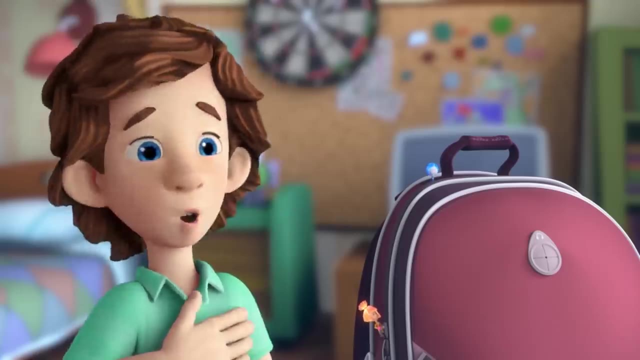 Ahh, I see, Nolik, where are you? There's work to do. I won't do it. I'm not gonna help such a greedy boy. Nolik, won't you help me out here, And I won't be so greedy anymore. 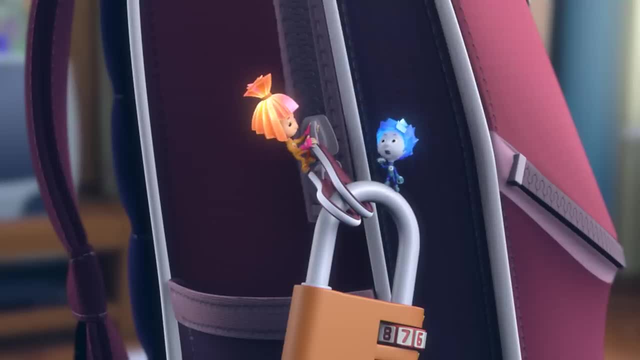 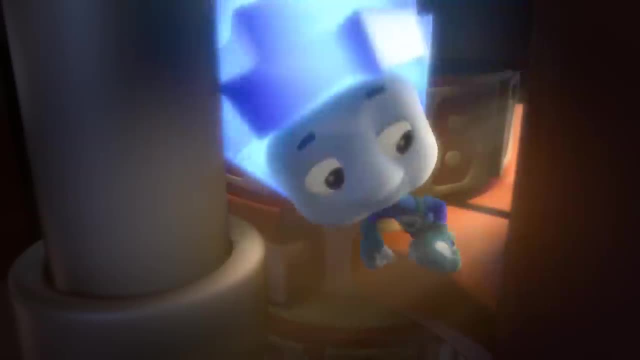 Alright, You broke me down. Omi, as soon as we're done, you're going to let me play with the game. Right, There's no room in here. Hang in there. We'll start turning the disks, one at a time. 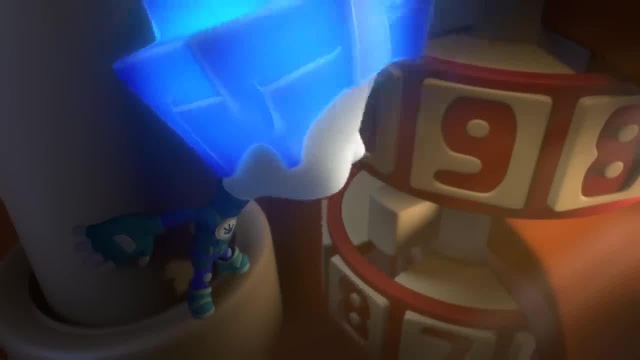 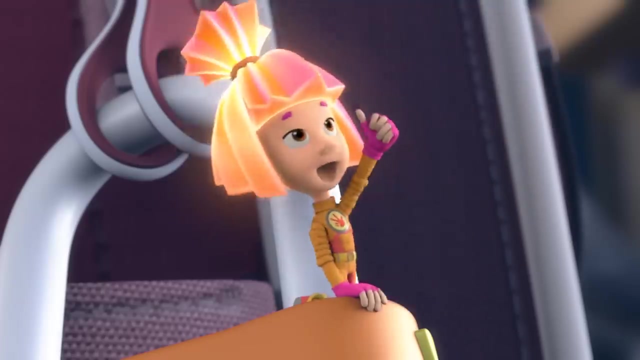 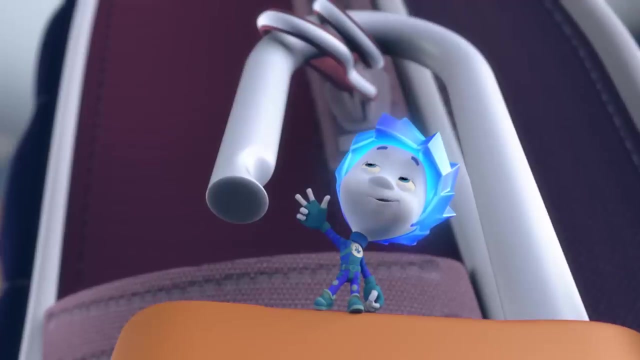 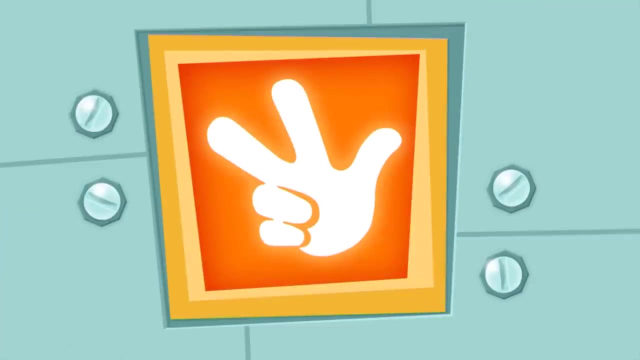 and you yell stop when they're lined up, Stop. Turn the next one now. Stop, Stop, Now try. Yes, Alley-oop Tideesh Hurrah. And your code was really simple, Way too simple. The secret numbers and letters that you use to lock something up. 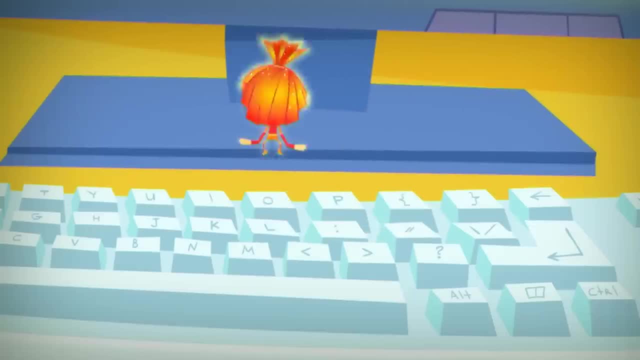 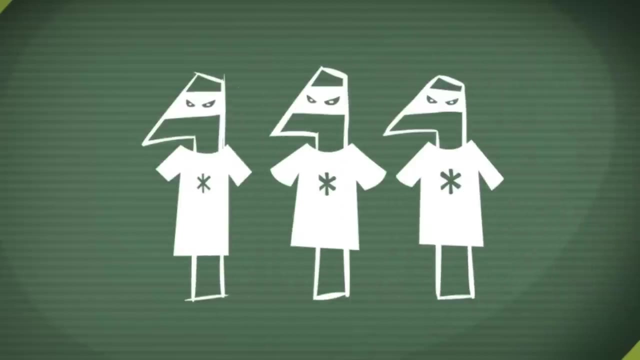 are called the code or the password. And to make sure your password is a really good one, here are some things you should know. Never choose a password that's really simple for someone else to guess, Like one with numbers or letters Or letters that are all the same or are all in order. 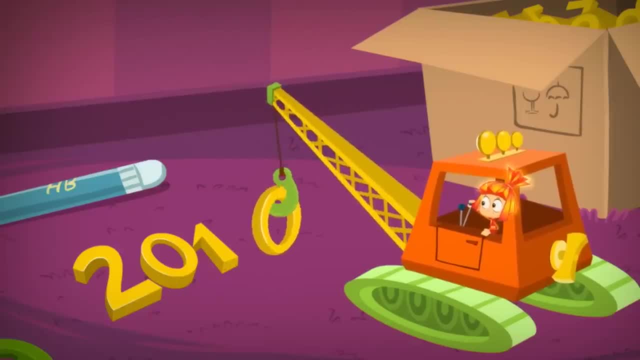 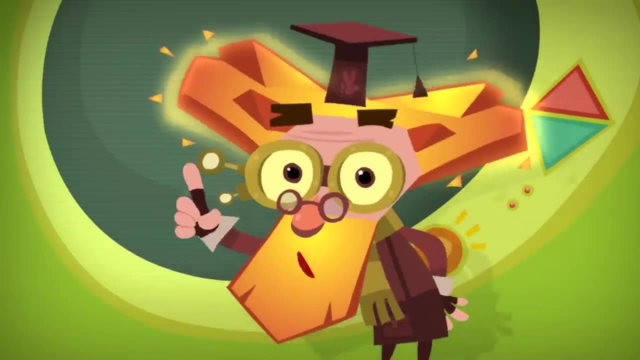 It's also a bad idea to make a password out of your birthdate or name. It's better to think of a password that's a bit more complicated, And don't forget your password once you come up with it. Write down your password on a piece of paper and keep it in a safe place. 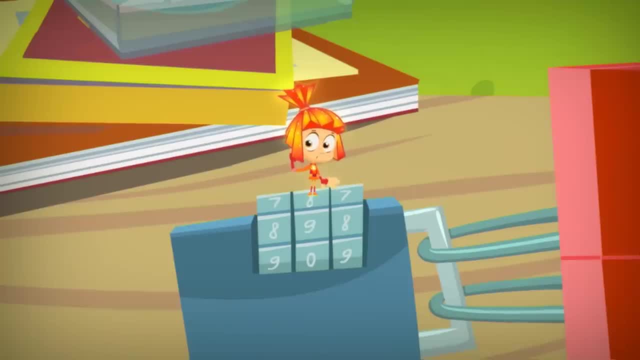 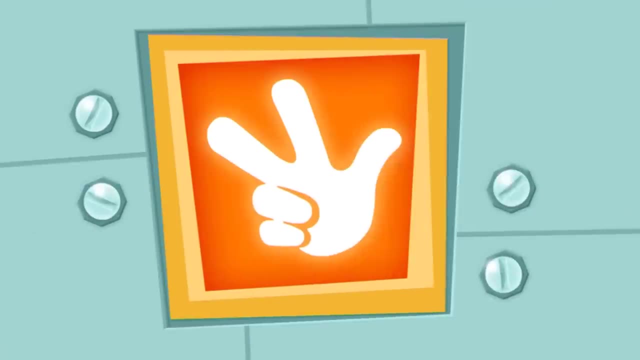 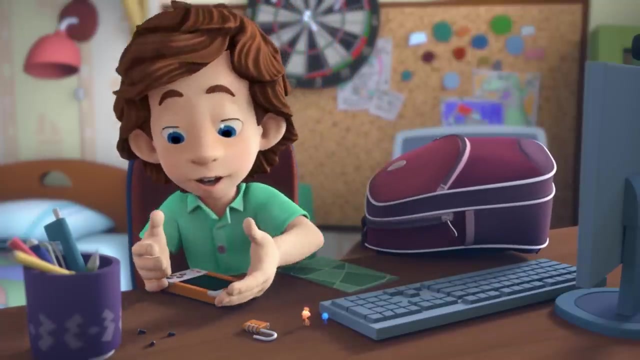 but don't show it to anybody else, And then, if you happen to forget your code or password, you'll be able to remember it with the help of that piece of paper. See you next time. And why did you ever put a lock on your backpack? 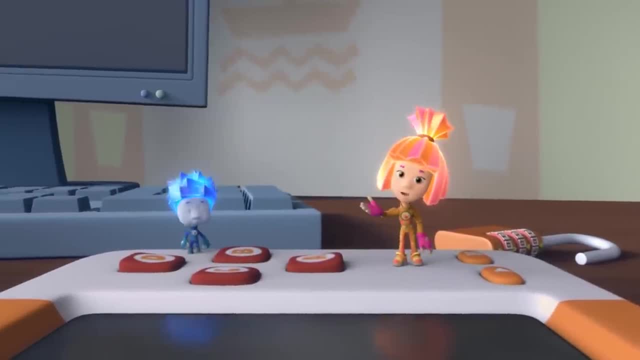 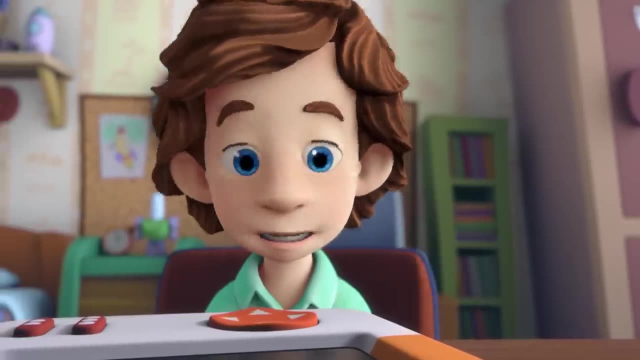 I was hiding the game from the other kids, Then why did you take it to school today? I wanted to show it off to my class And did you show it No way? If they would have seen it, they'd be like: 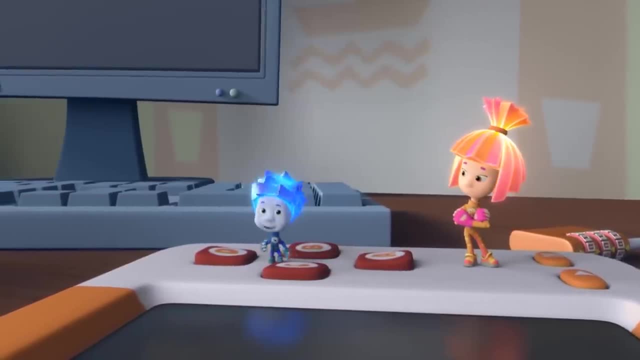 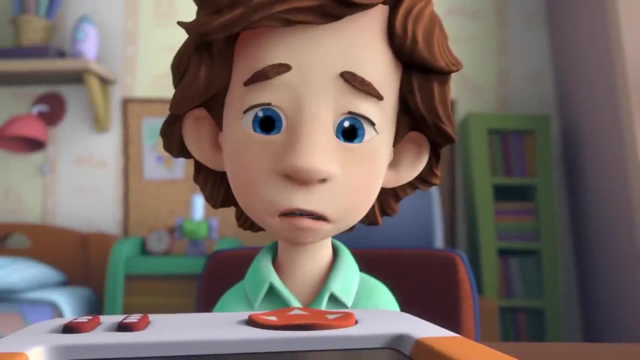 I want to use it, I want to play, And so you hid it and didn't show it to anybody, Not to anyone. Then why take it to school silly To show it off there? You're just some show-off. You're just some greedy…. 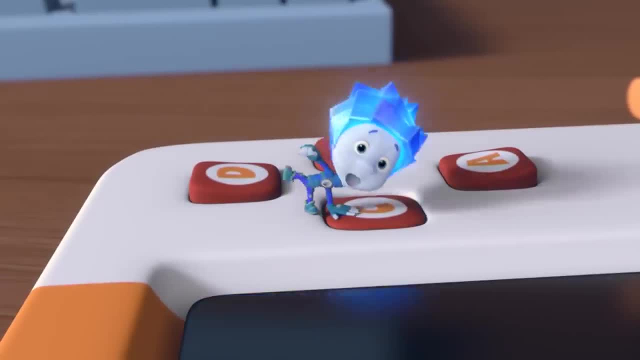 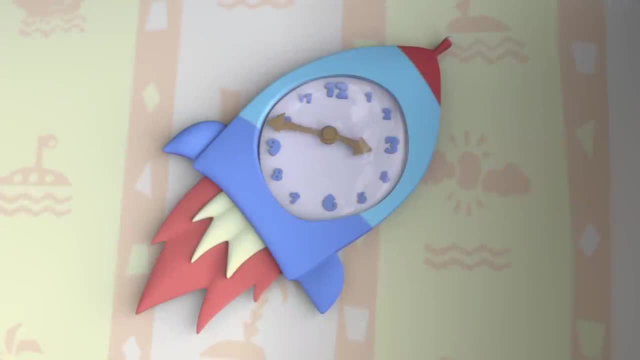 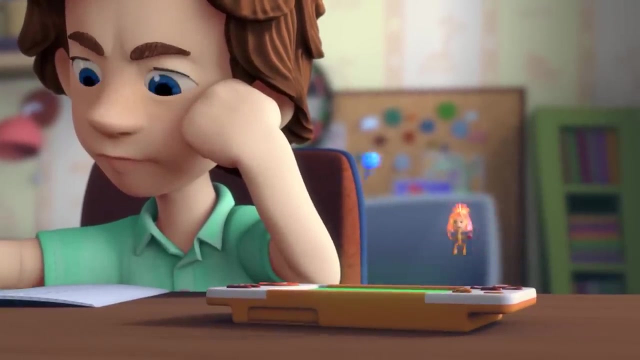 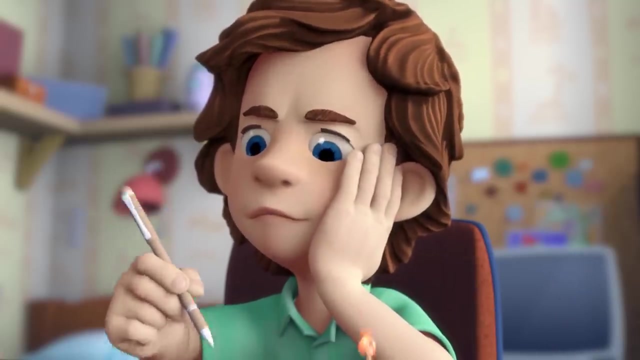 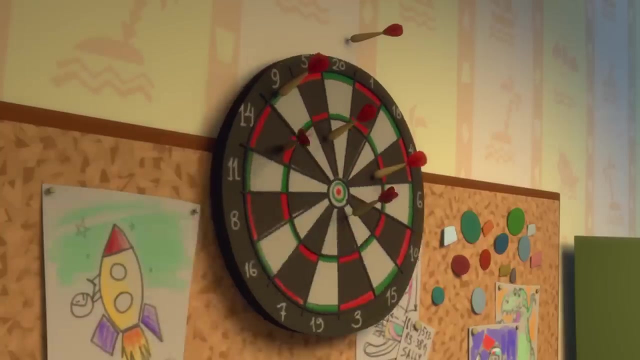 Oops, Sorry Once, greedy boy, Will you let us play now Play away. We're not bothering, you are we. Can you jump a little easier? You're shaking the whole desk. You'll miss for sure. No problem, Anybody can do that. 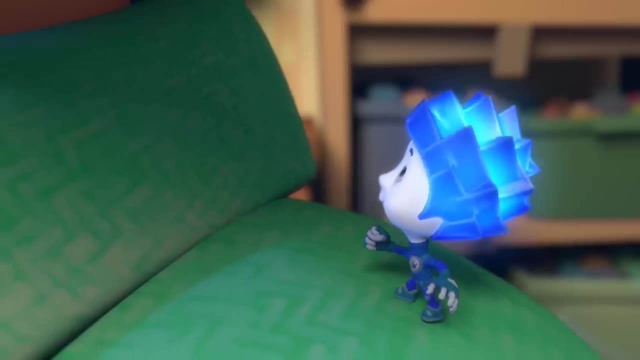 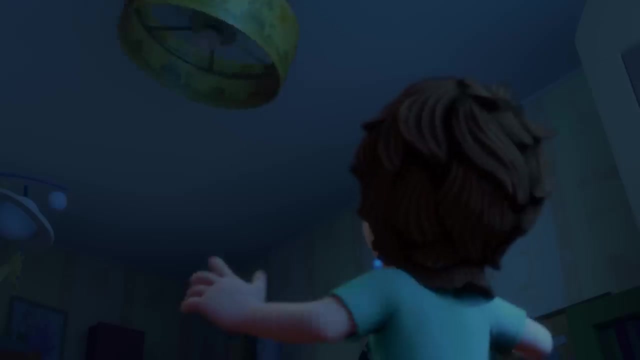 But I bet you can't do it if you tried bouncing the ball off the floor first. Just look, What are my parents going to do to me. Maybe we should call Simka Simka. And what's Simka going to do to us when she sees this? 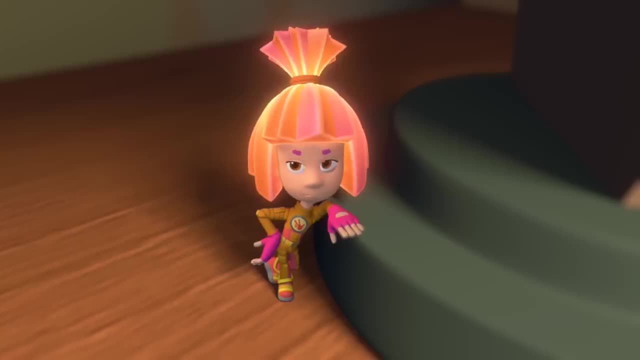 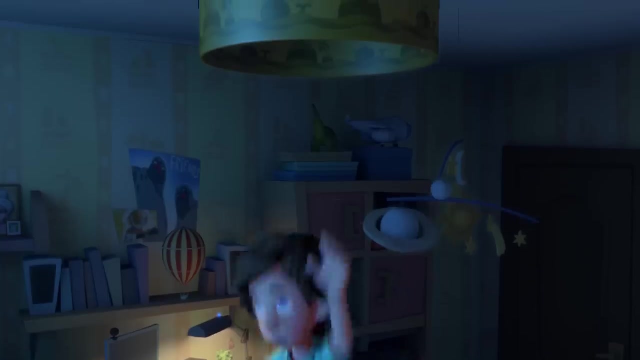 So got yourself in trouble. huh, You shouldn't be playing with a ball inside, And now we have your lamp to fix. But how? Only my dad can reach all the way up there. Why, just your dad? You have a hot air balloon over there. 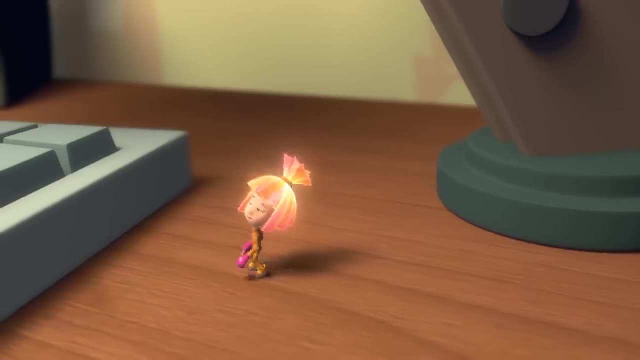 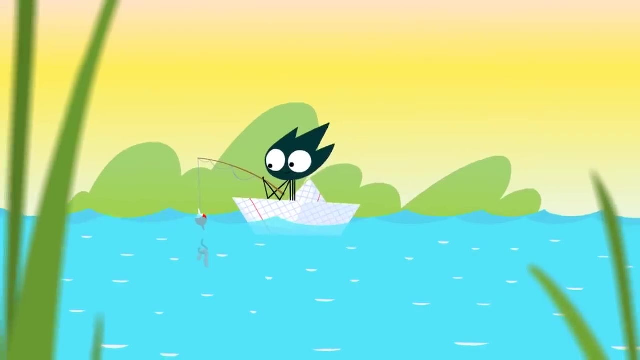 That doesn't fly, It's just a toy. see, Well, it might be just a toy to you, But for us Fixies, it's absolutely real. Let's see what it can do for us. If an object is lighter than water, it floats up to the surface. 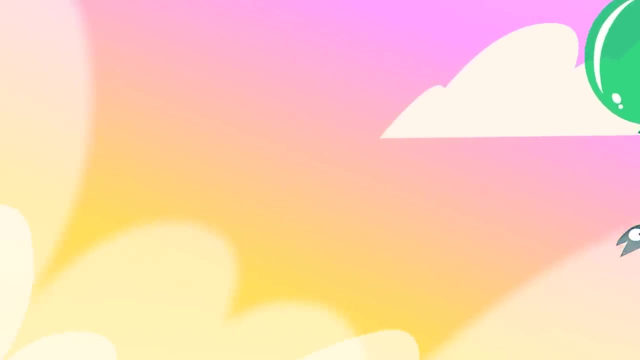 And in the same way, if something is lighter than air, it floats upward. Did you know that hot air is lighter than cold air? Well, it is, And that means, if you warm up the air in a balloon, it will float up. 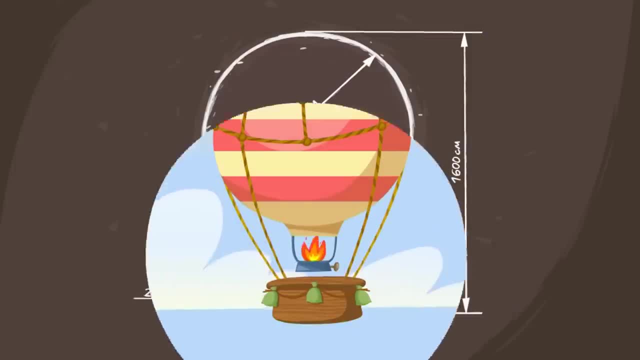 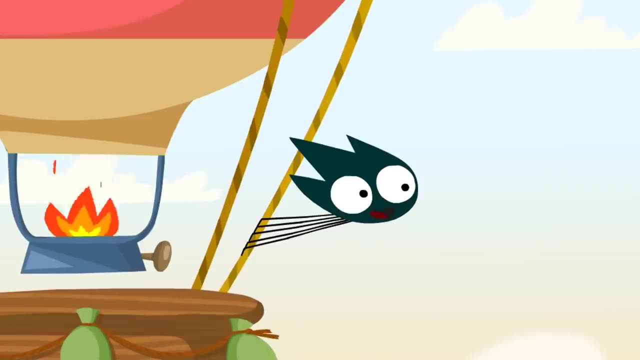 Hot air balloons use special gas burners to heat up the air inside of them, so they will get lighter. And the bigger the balloon, the more people it can take up to the surface, And that's why it's called a hot air balloon. 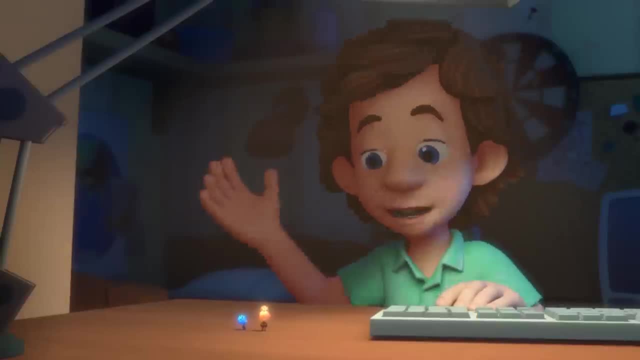 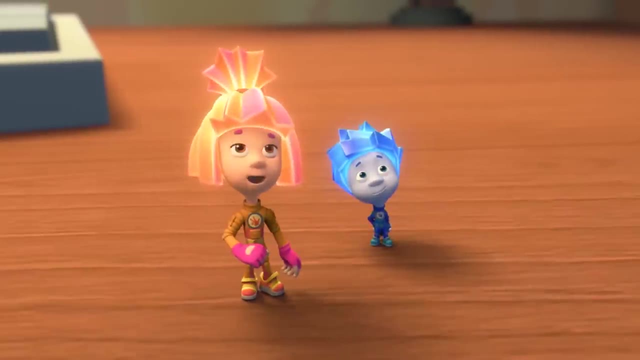 It can blow up into the air. I know what you're saying, but where do we get a burner? You think Fixies don't have their own burners? Ha, Sure, we've got them. Bring it down here and I'll go talk to our parents. 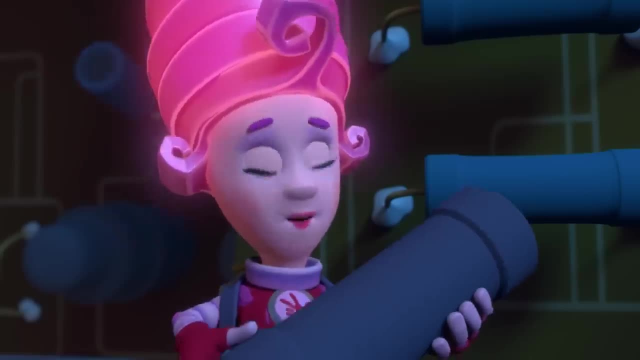 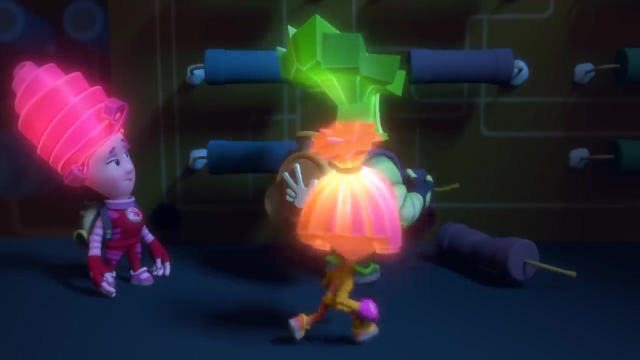 No, no and no. The human child must never see us. Listen now, Simka. We already don't approve of him seeing you and Nolik, He won't look. You're the one who told us how you dreamed of flying. 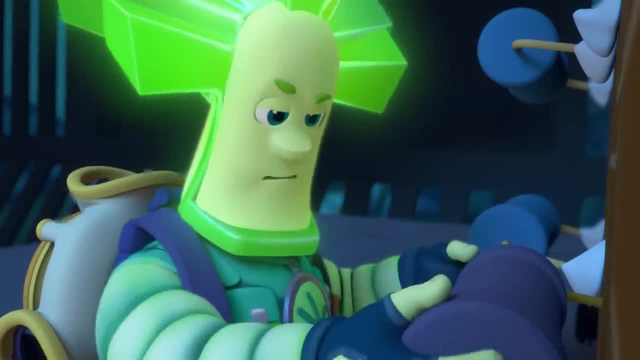 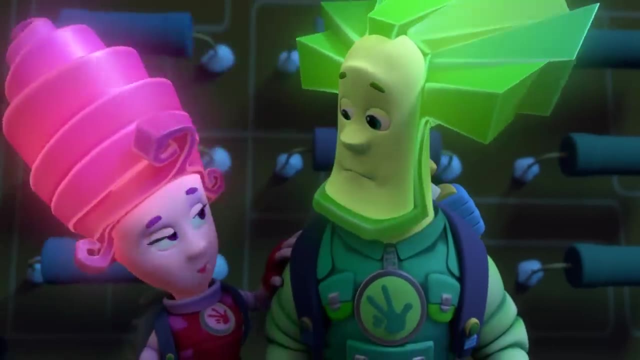 since you trained to go into space? Yeah, For two years I waited on standby, but I never went up, And you've never flown on a hot air balloon either, honey. So let's call it a deal. I talked them into it. 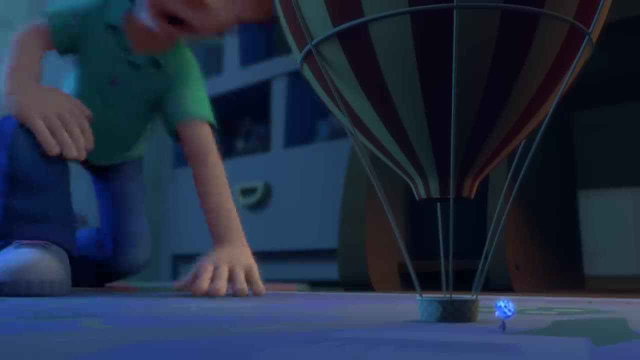 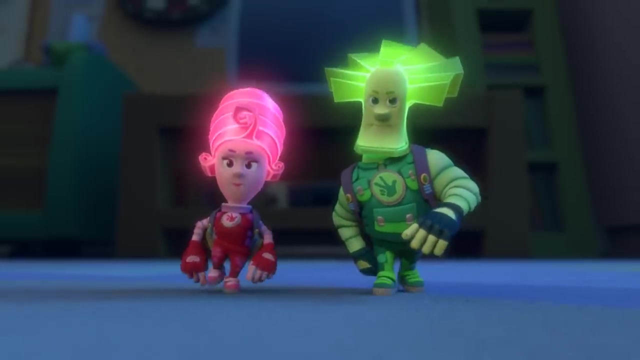 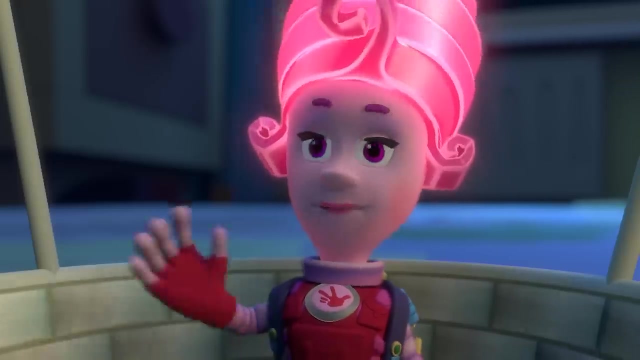 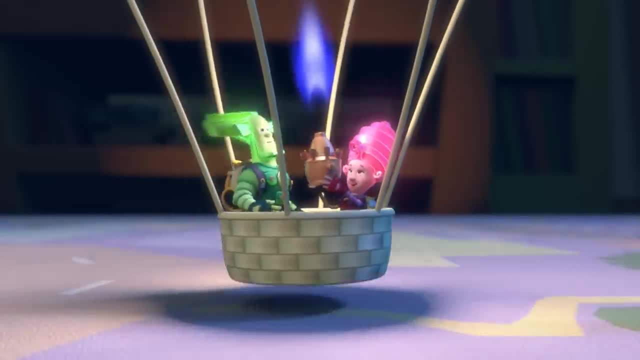 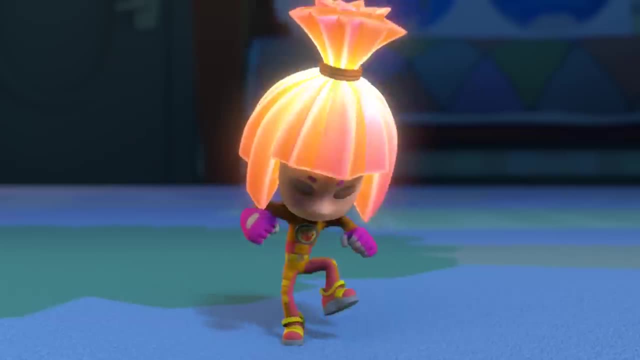 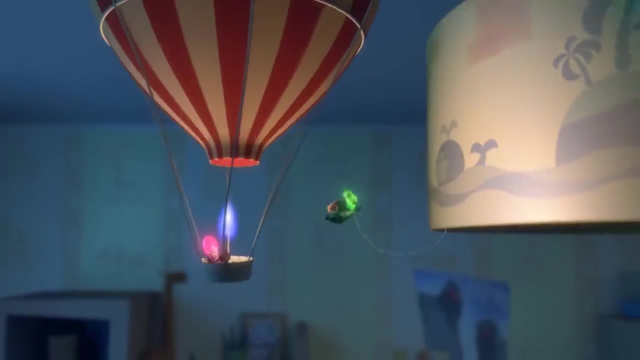 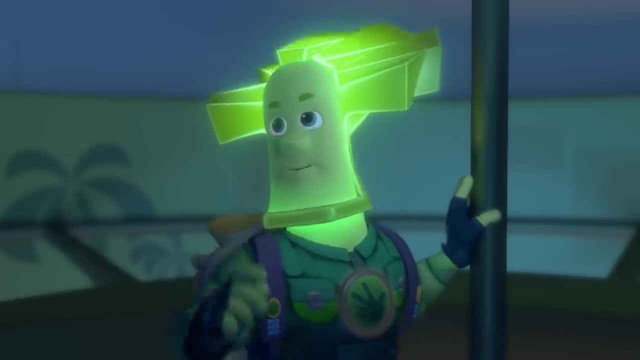 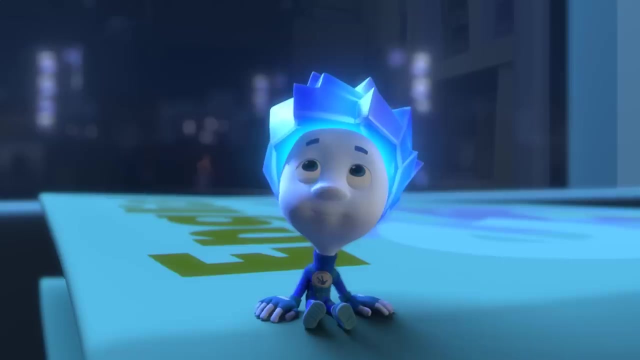 Permission is granted And off we go. Hooray, It's flying, Don't you peek, Turn around. Oh, it was an accident. I'm going to evaluate the damage, Maintaining proper altitude, So they've reached the spot. 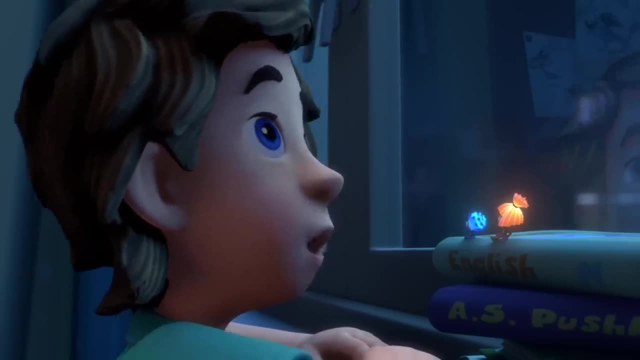 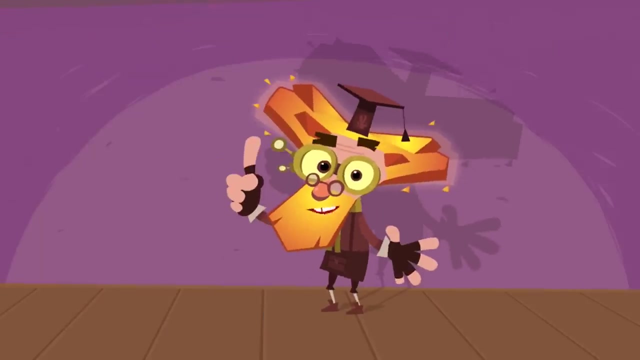 Air balloons are really awesome. I wonder who figured out how to do that. It was the Montgolfiers. The hot air balloon was invented in the 18th century by the Montgolfier brothers from France. In those days there were no gas burners. 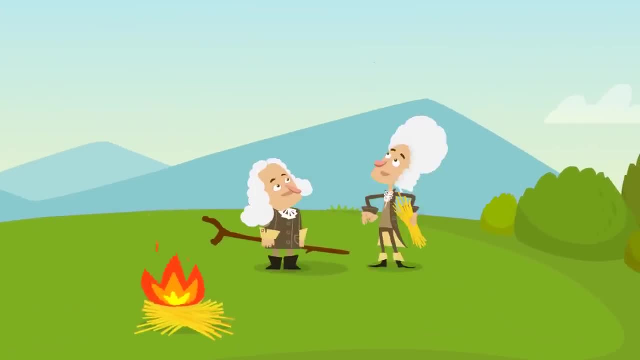 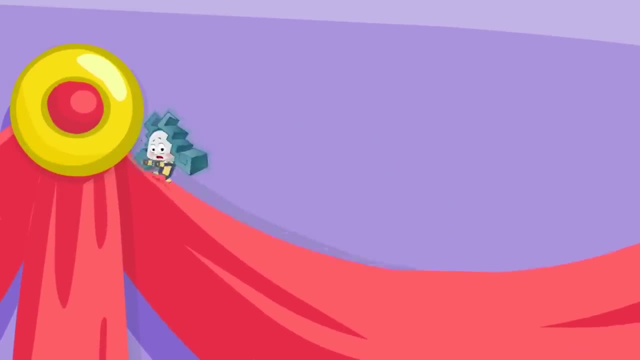 So they heated the air inside the balloon by burning straw. At first there were no passengers on their balloon, Not counting the Fixies, of course. I mean how else could a balloon get up in the air without them? Unfortunately, the names of the first Fixies who took that flight. 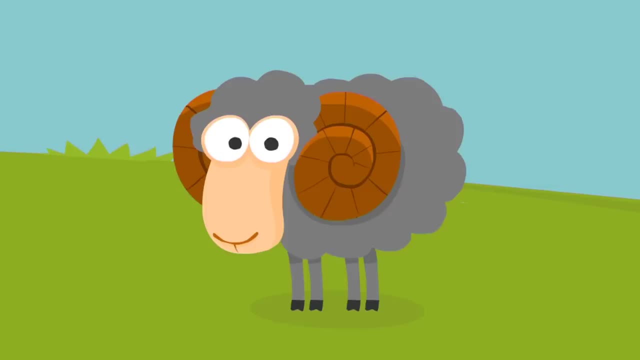 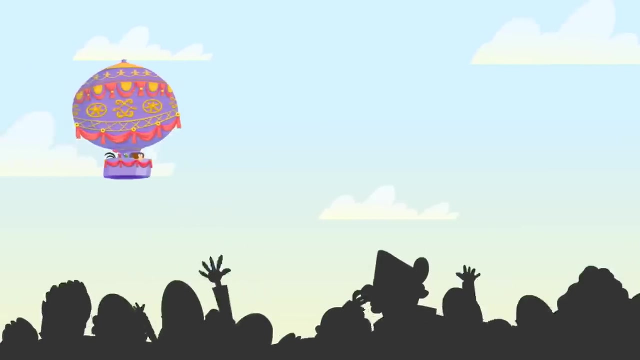 were not recorded in the annals of history. Following the Fixies' flight, the next passengers were animals: A ram, a rooster and a duck- And it was not until those two people who were on the air balloon safely landed after flying a full four kilometers. 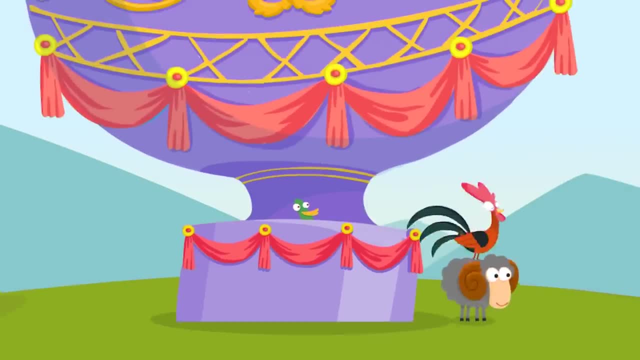 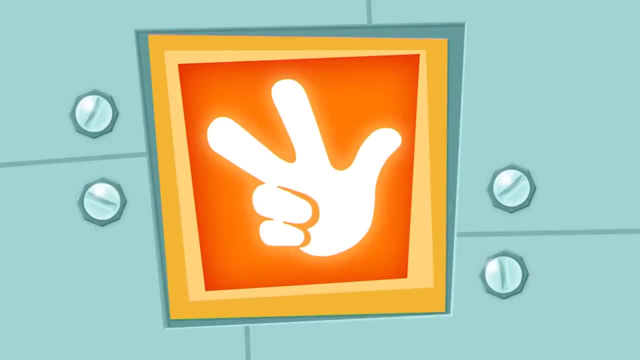 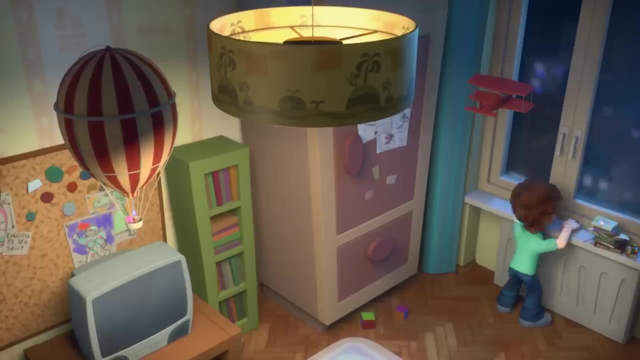 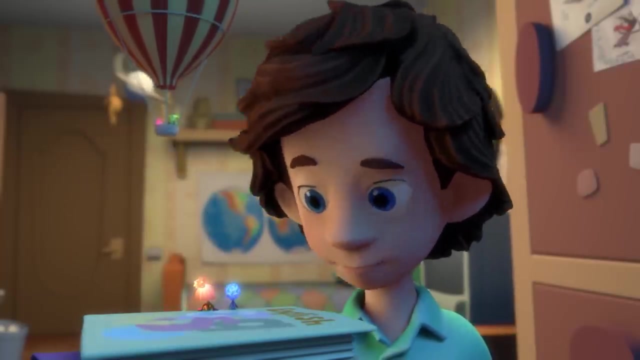 that humans dared to fly in hot air balloons themselves. Ever since their invention, hot air balloons have also gone by another name: Montgolfiers, Hurray, Tideesh, Tideesh. All right, Simka, please let your parents know that I'm so. 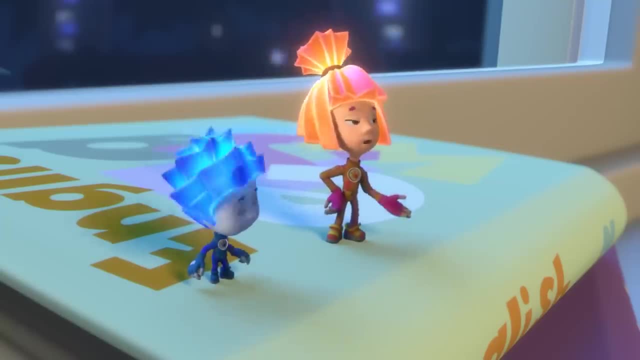 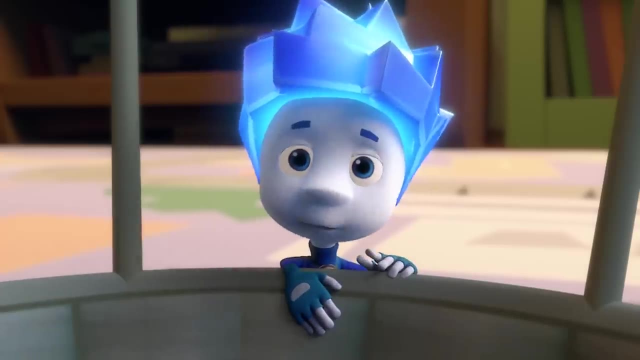 Simka, please let your parents know that I'm so Simka, please let your parents know that I'm so very thankful. Okay, By the way, now you can turn around. You know, Simka? let's fly the balloon, just like them. 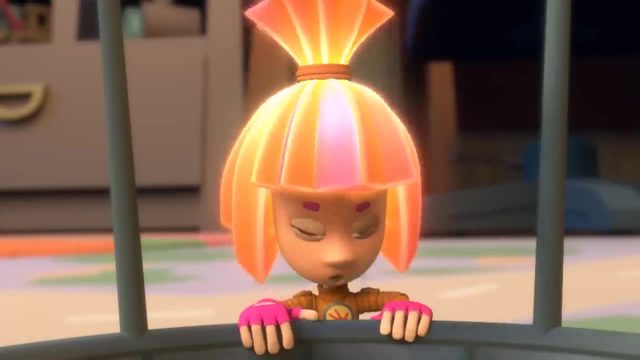 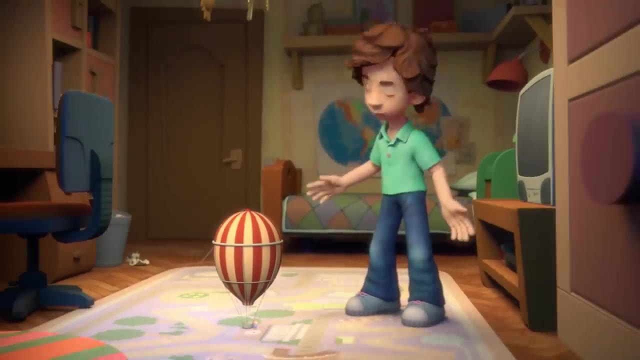 There's no way, Nolik. We would need to use the burner, And kids aren't allowed to play with fire. I'll give you a ride. Look, I still need to put it back up on the shelf, So climb in and let's do it. 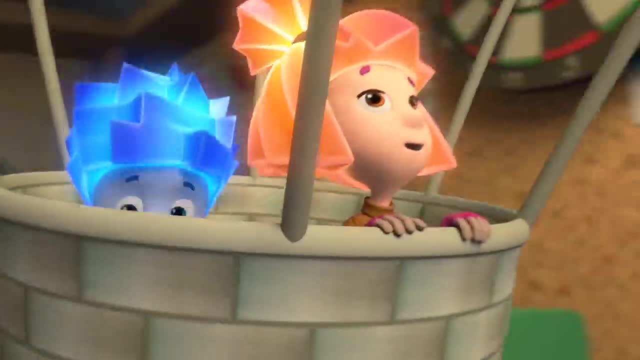 Ha-ha. Oh yeah, This is great, Simka. Look at us, We're flying just like the Montgolfiers brothers. What do you mean like brothers? Okay, then, Like brother and sister Montgolfiers. 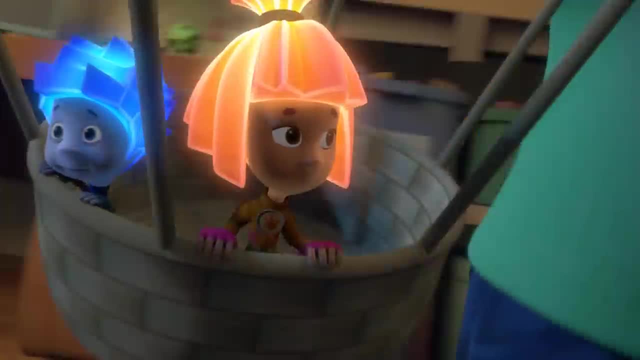 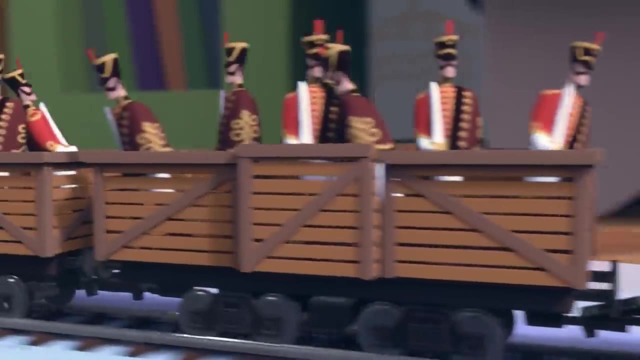 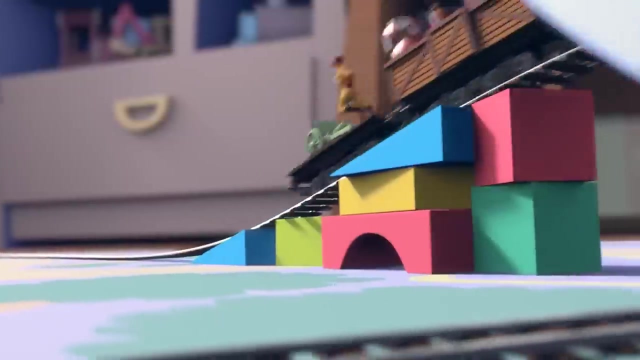 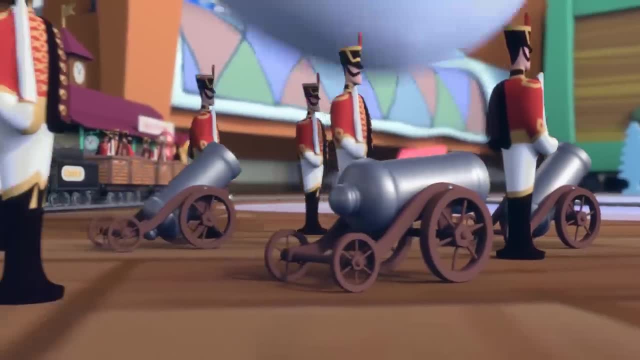 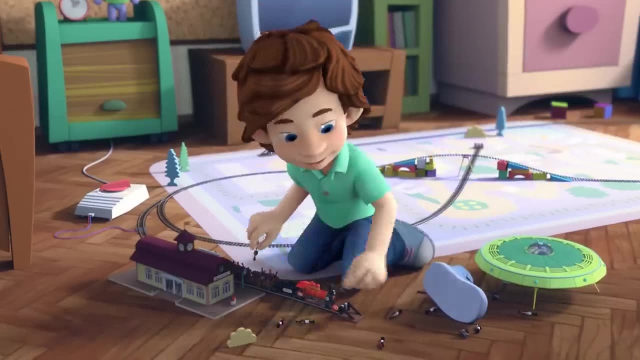 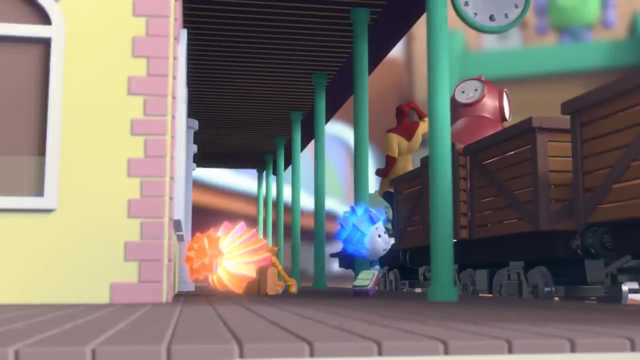 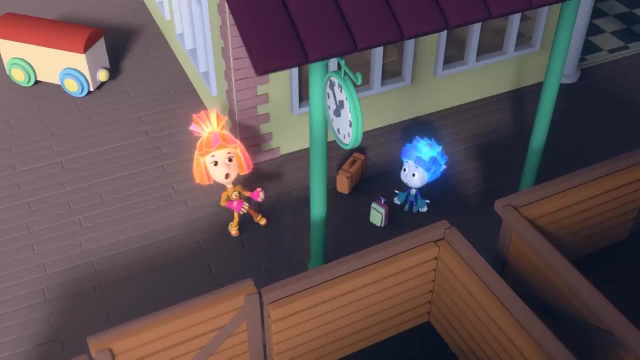 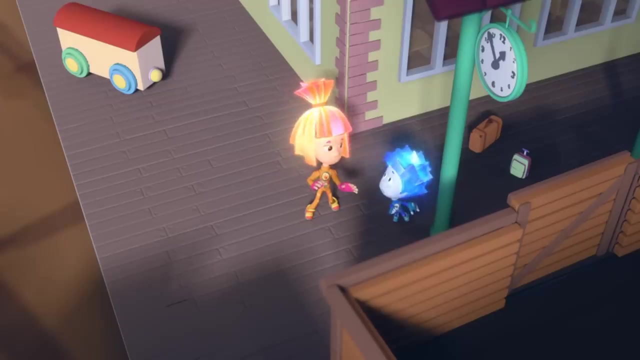 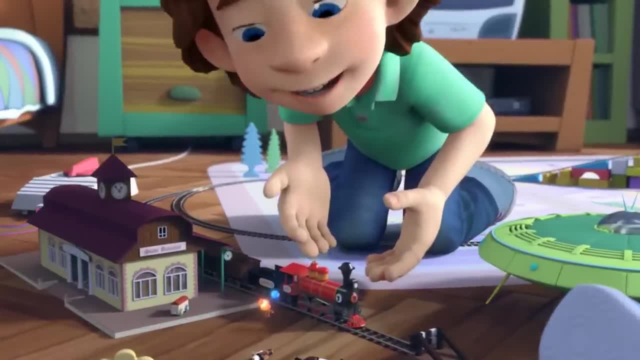 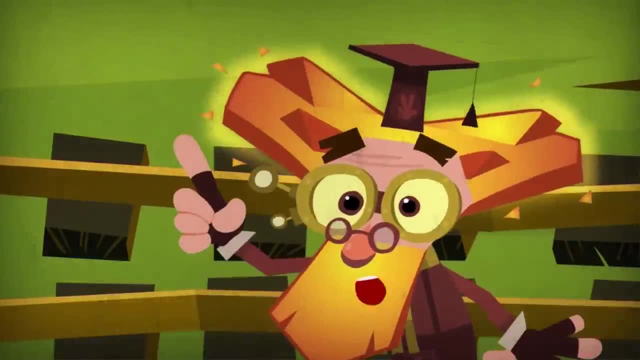 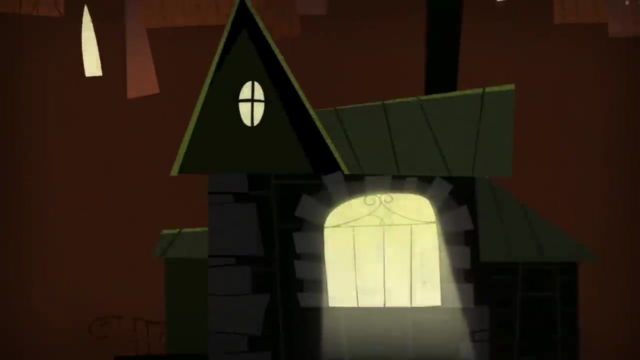 Train engineers. You don't know anything about driving a train. Oh, we know plenty about trains. Humans invented the railroad long ago, but back then the rails were made out of wood. People didn't start making metal rails until the end of the 18th century. 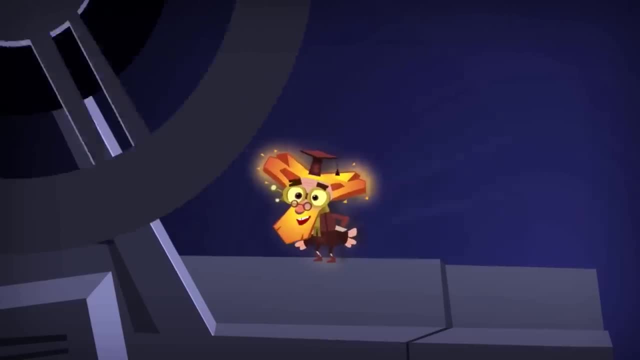 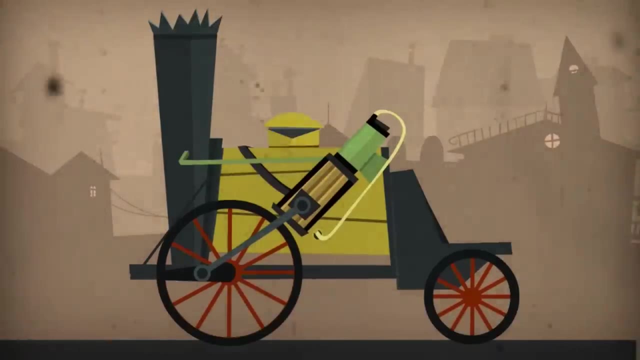 But the first railroad cars had no engines to give them their power. Instead, they used horses to pull them along. Later, horses were replaced by the steam engine. Wood and coal would burn in their furnaces to boil the water in the boilers. 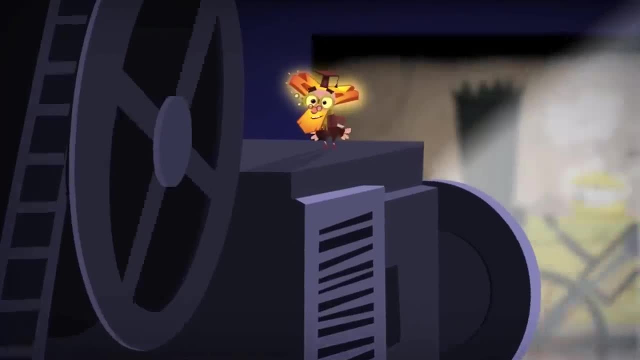 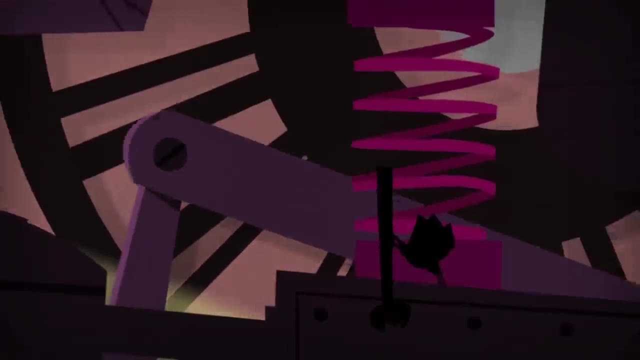 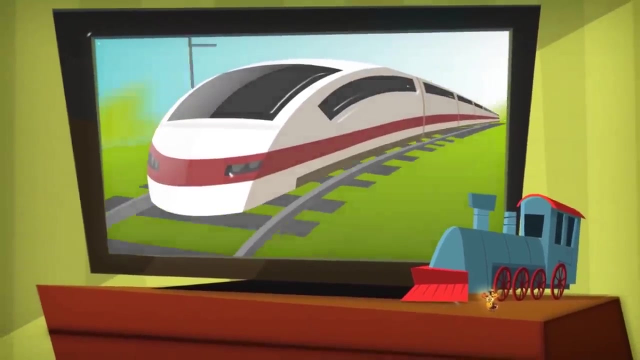 making the steam that turned their wheels. And the Fixies were there to help those trains go, making sure all of the parts could work together smoothly. But now steam engines have long gone away. The railroad uses electricity now for its power. These electric trains race along the railway. 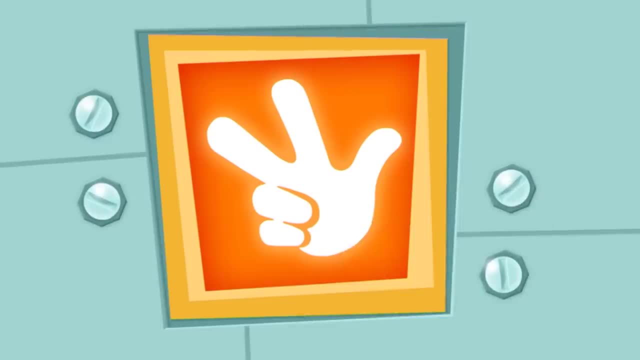 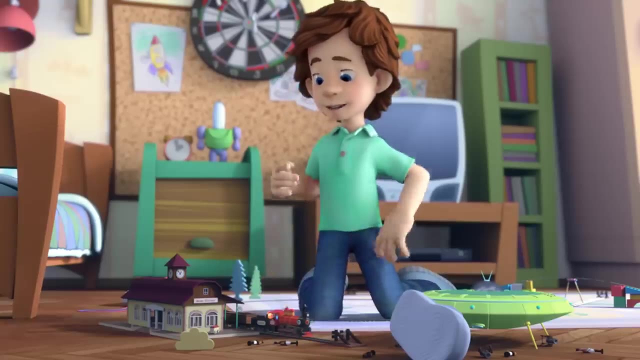 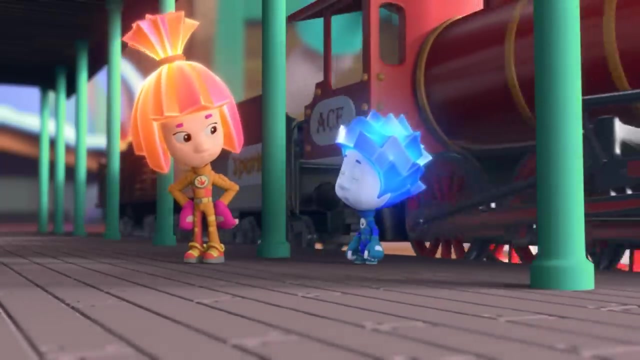 at almost the speed of an airplane. So you might know trains, but you'll still be the aliens. This railroad is mine, so you're gonna play the way I want. The train is unloaded and, leaving the station, You can play choo-choo by yourself. 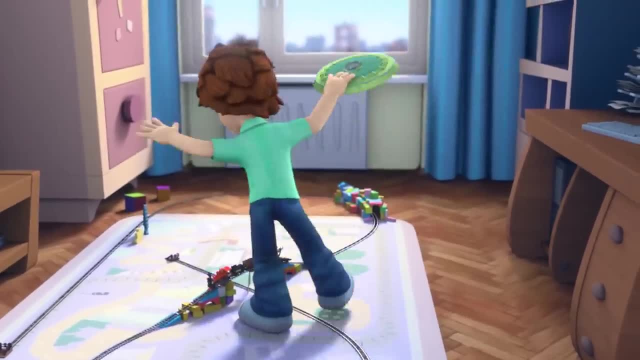 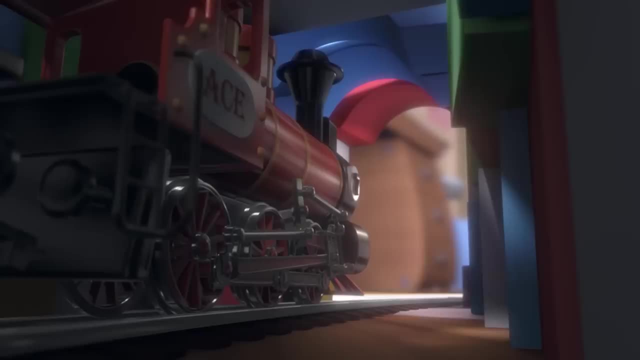 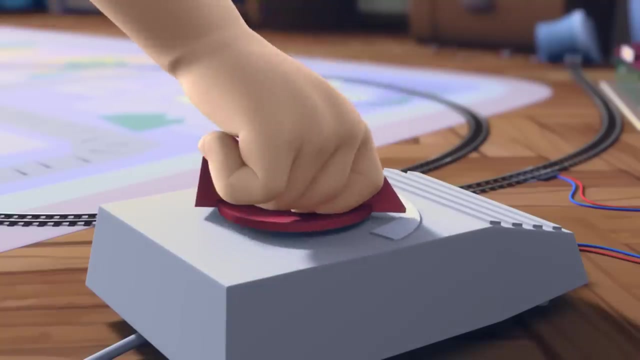 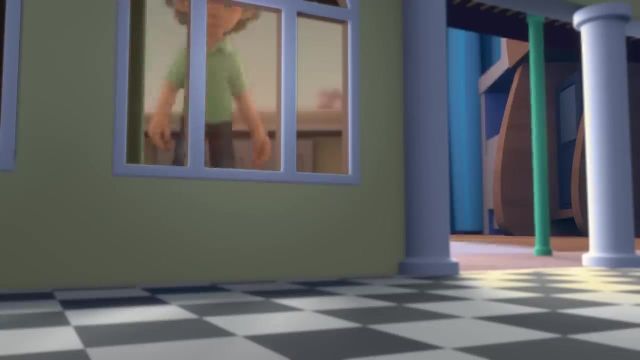 And I will Choo-choo, choo-choo, Choo-choo. Hey, why did you stop? This doesn't help either. It's not going at all. Simka Nolik, Where are you? 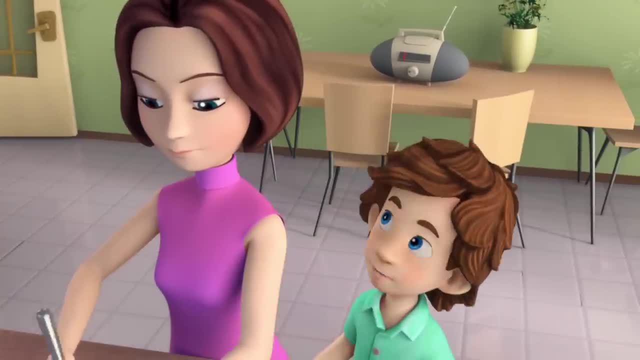 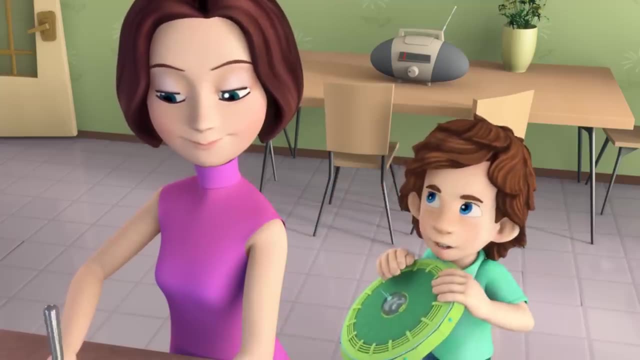 Did I hurt your feelings or something? Mom, is Dad gonna be home soon? No, Is something the matter? We've been attacked by evil aliens. The train has to be fixed right away or we'll never escape them. Uh, mm-hmm, You want some tea. 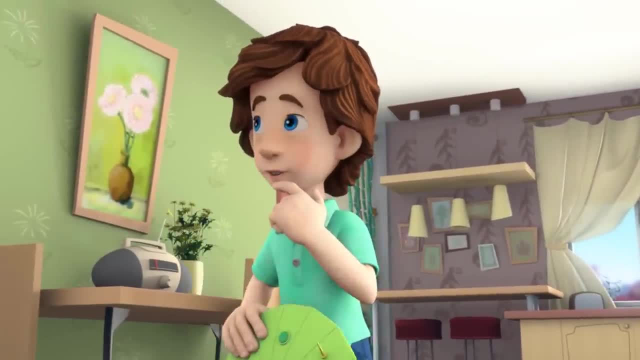 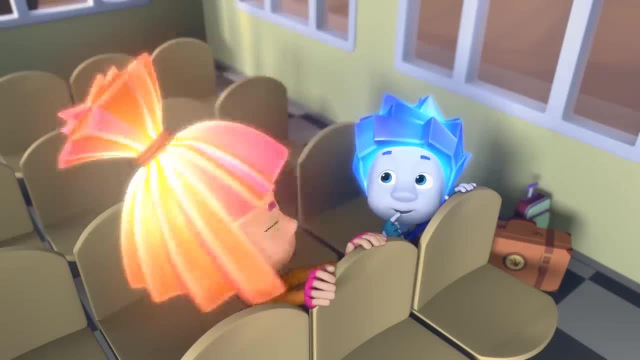 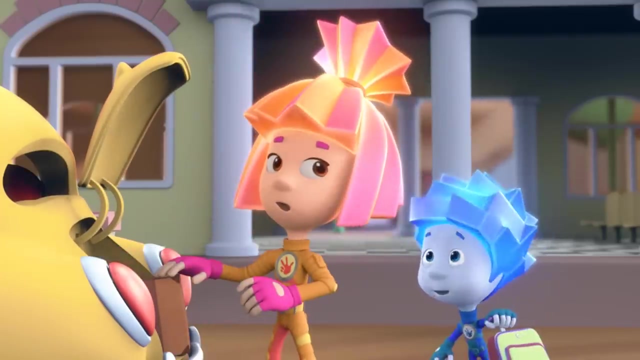 Ah, I've got to think of something. Simka Nolik, I know you're in there. Please forgive me if I hurt your feelings. I'm really sorry. There's nobody but you that can save the world from the evil aliens. 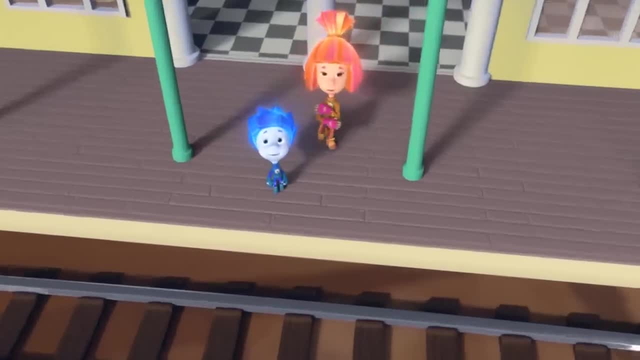 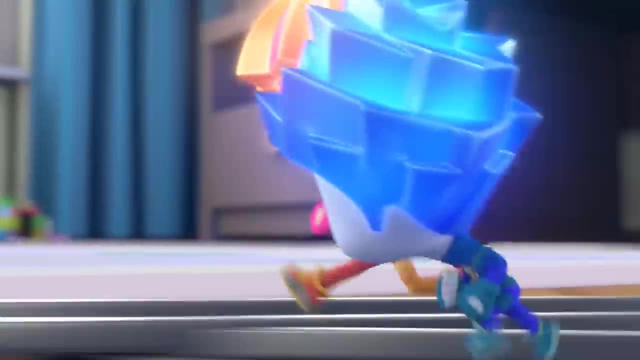 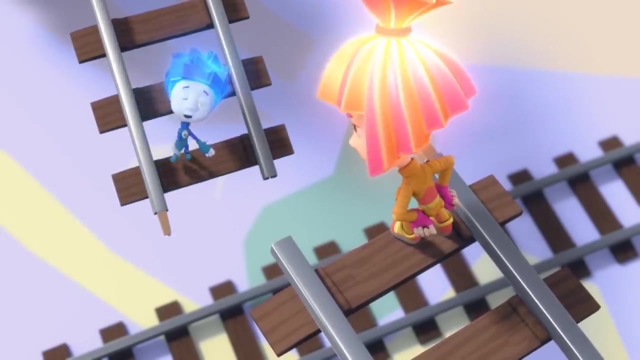 Pfft, Alright, It talked us back into it. Well, let's go and check the rails. Nolik, follow me, I'm faster, Whoa Well. so much for being faster, But it looks like I found the break. 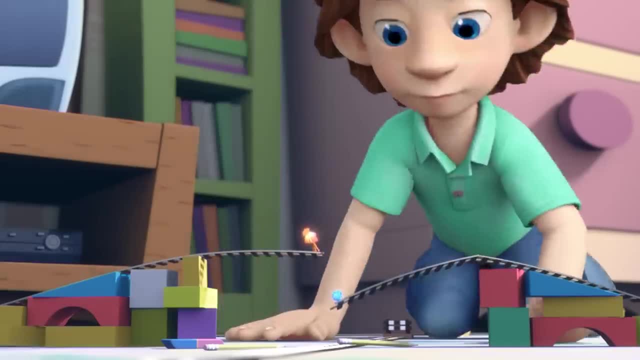 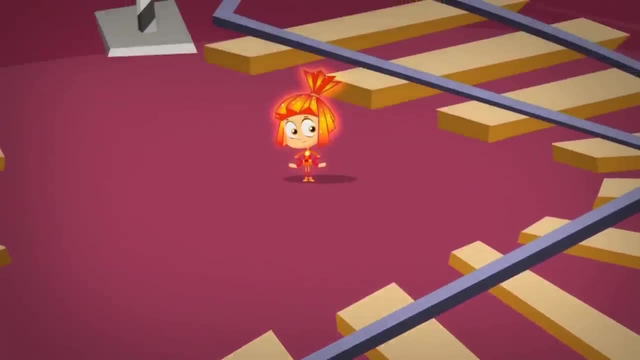 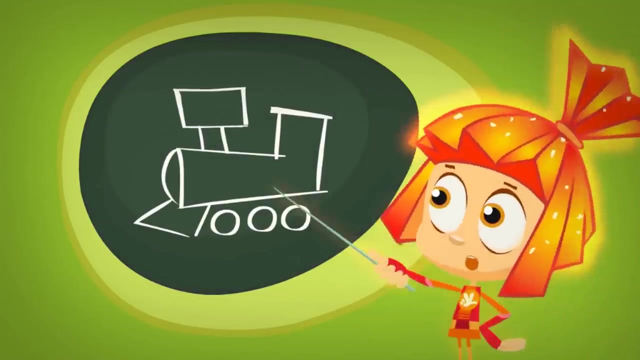 Tom Thomas, The rails are broken, I know, and so You know, but that's why your train's not running Just like a real train model trains run on electricity But there aren't any batteries inside the locomotive to pull the other cars. 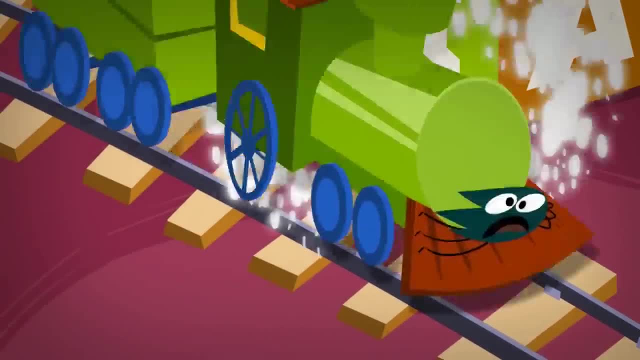 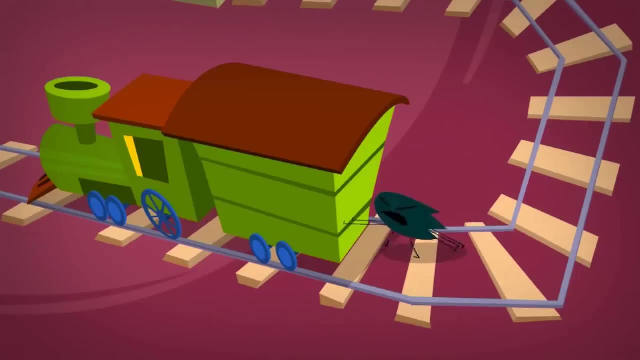 the engine gets its electricity from the rails. Each piece of the rail has a wire in it. If the rails come apart, the electricity can't flow through the track and get to the train, And without electricity the train's engine just stops going. 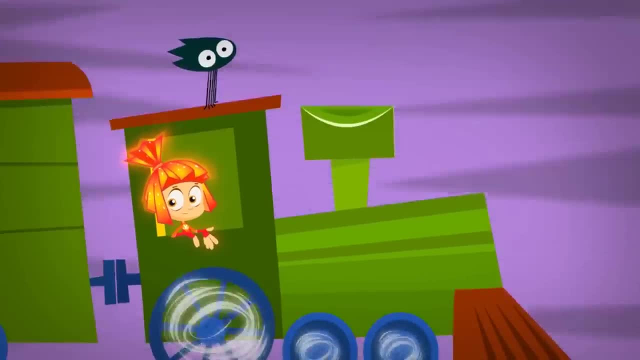 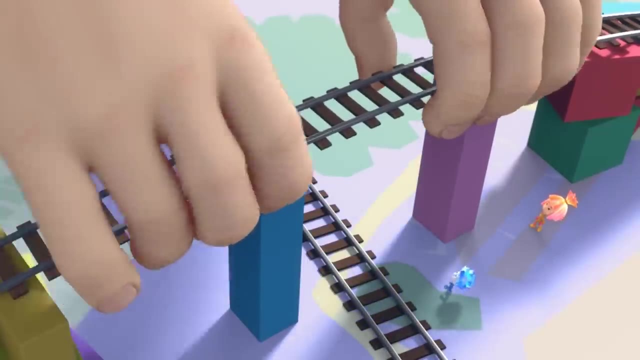 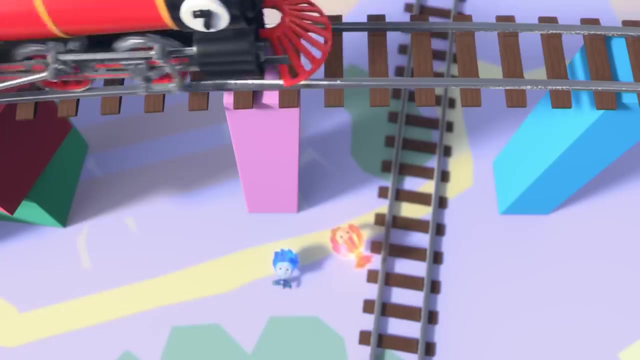 So reconnect the rails and your train will run again. Ah, Uh-huh, put them together. Ah, yes, Hooray, the train's running Way to go. So will you play with me now? And which way are we playing this time? 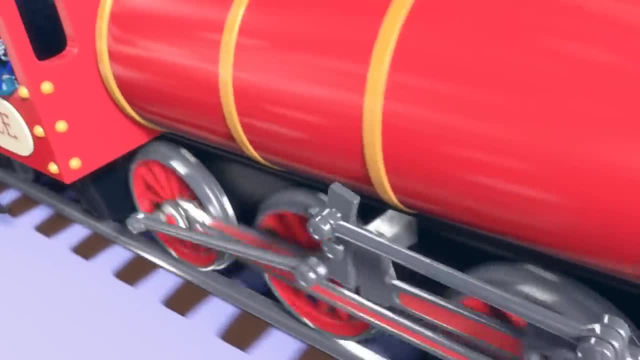 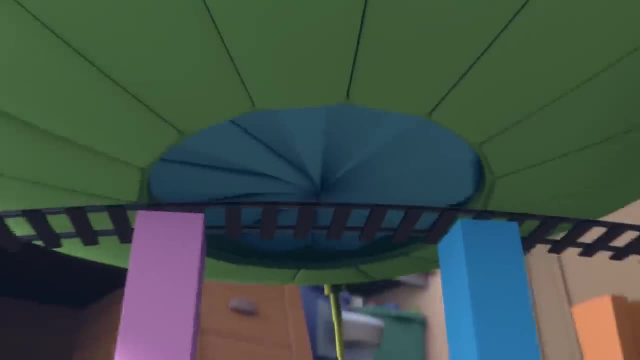 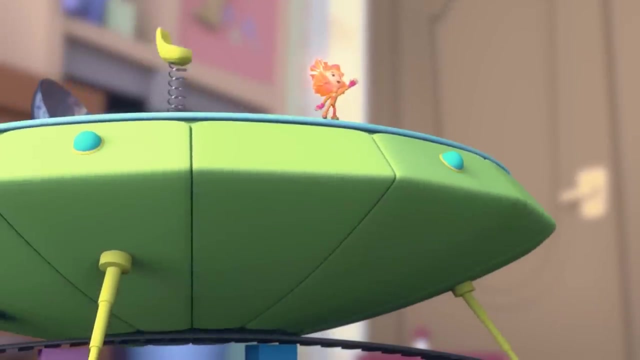 Whatever you want, I'm with you. The train rushes down the track, with no luck as its engineer. when suddenly from out of the sky comes an alien spaceship, I'll be right back. Greetings to you, oh people of planet Earth. 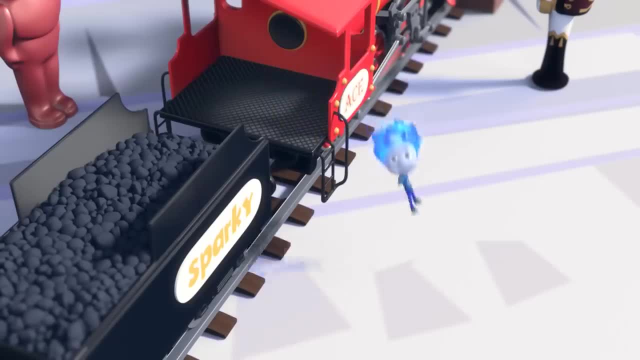 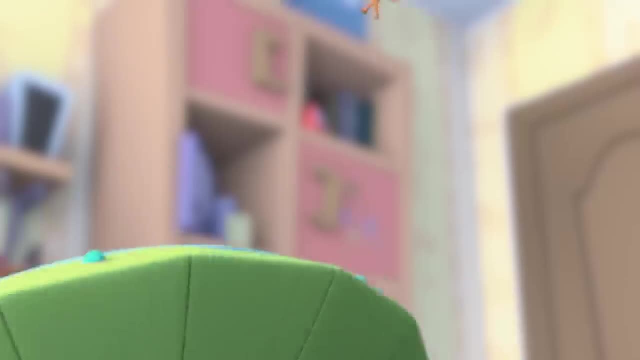 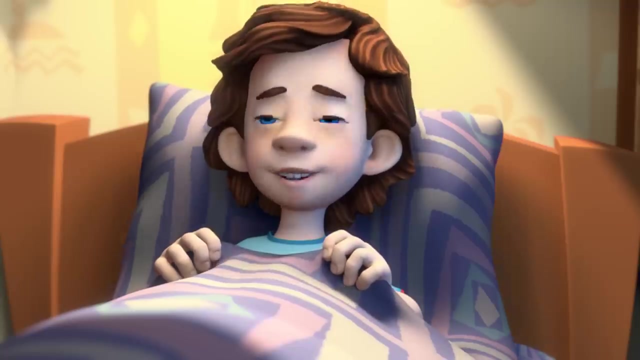 I come from far away, from another galaxy. Have you come to destroy everything? No, I've come to fix it all. Oh Yes, honey, only a thousand times or so. A robotazoid R300 would just be the greatest. 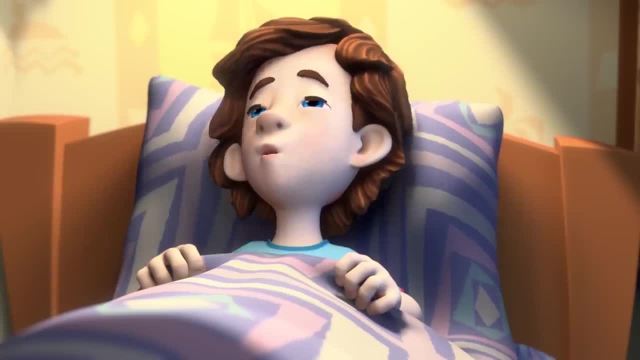 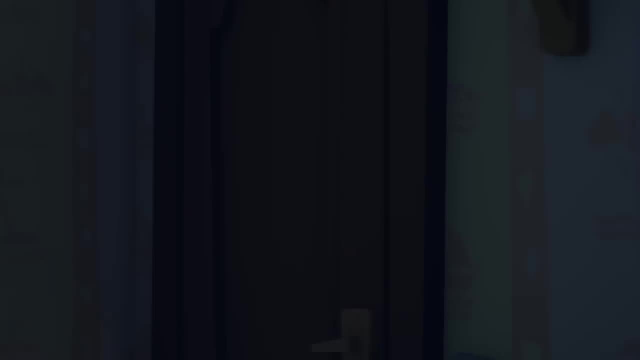 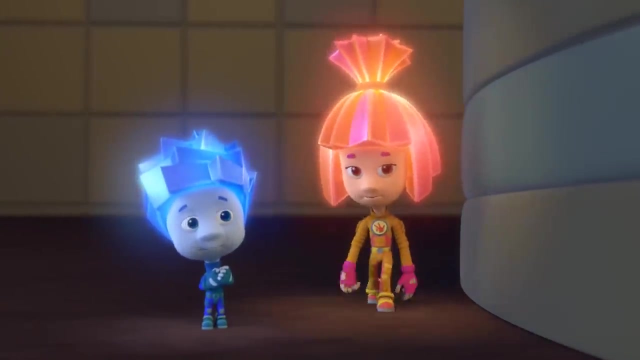 With mega vision. I want it, I really do. I do. Well, tomorrow you'll find out, But now it's time to sleep. Tom Thomas, Wow, that is one great present. And we got Tom Thomas absolutely zero for his birthday. 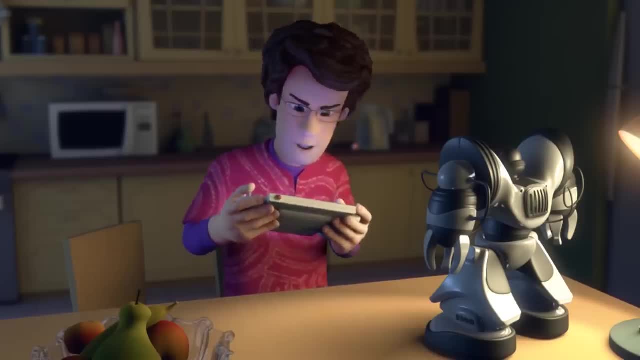 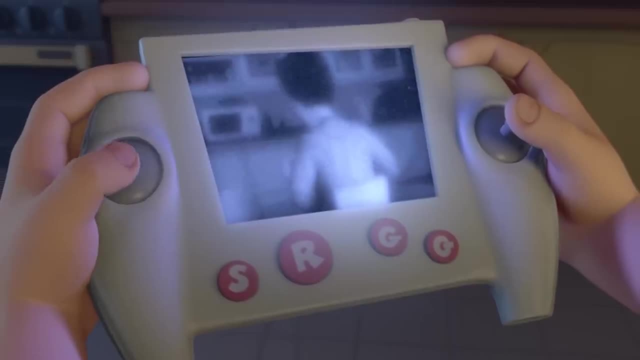 We're just terrible friends. So how does this robot work? OK, so let's give this a try, shall we? First we'll take a walk, And how does he have any idea where the robot is going? I can tell you. 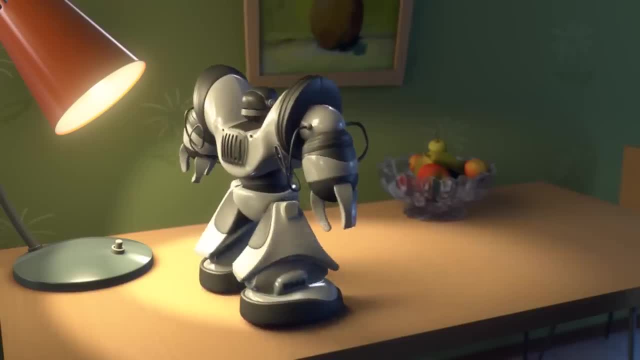 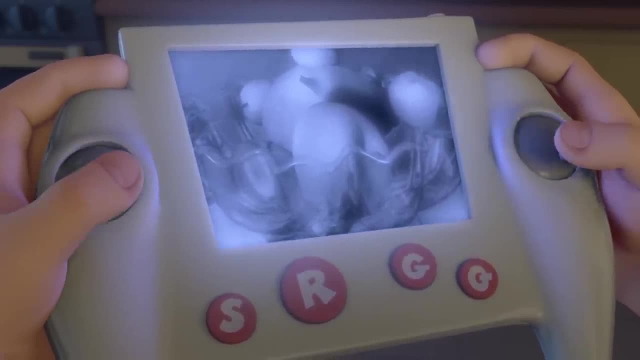 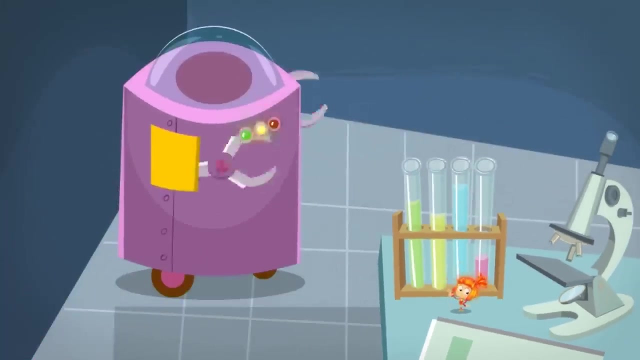 One of the robot's eyes is a video camera. The robot sends the picture to the screen on the controller so the player can see where the robot is going. Yeah, And that's just one thing they know how to do. A robot is a smart machine that can do very difficult or dangerous work for humans. 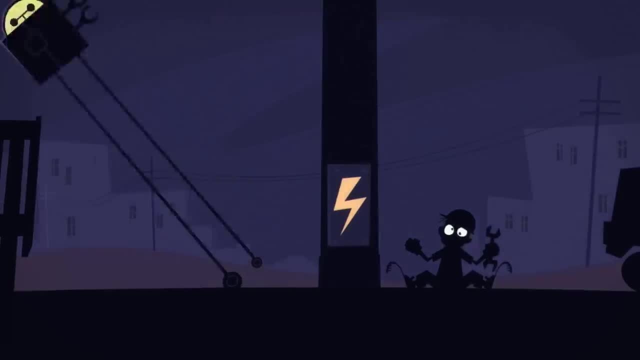 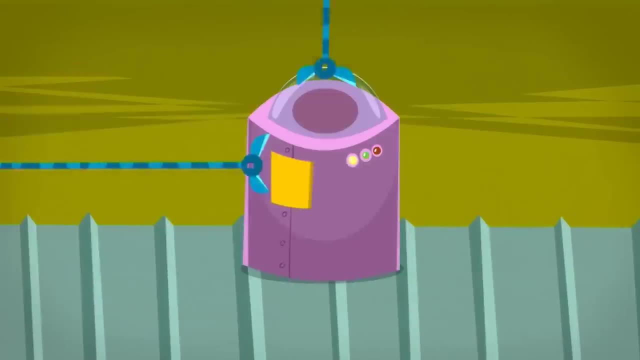 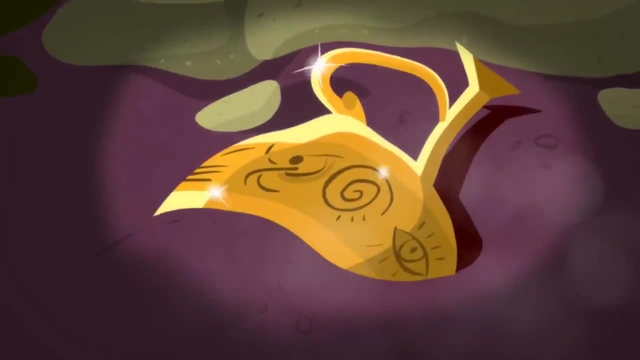 With its eyes it can tell you where the robot is going. With strong metal arms, a robot can move heavy objects or put together parts to build cars and other machines. Robots are often sent into outer space or to the bottom of the ocean to help scientists. 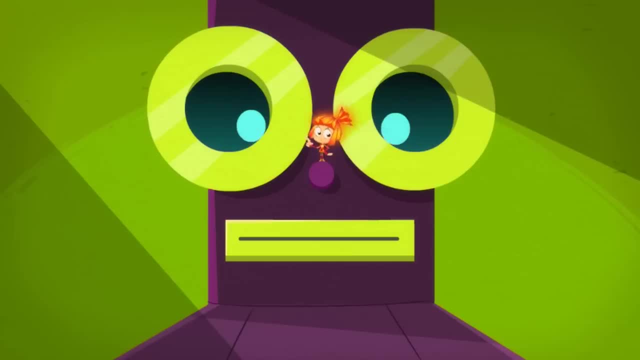 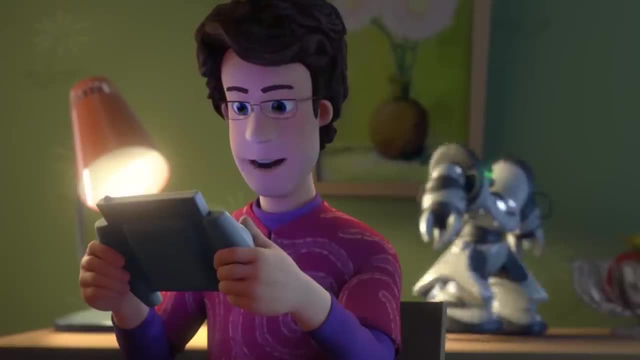 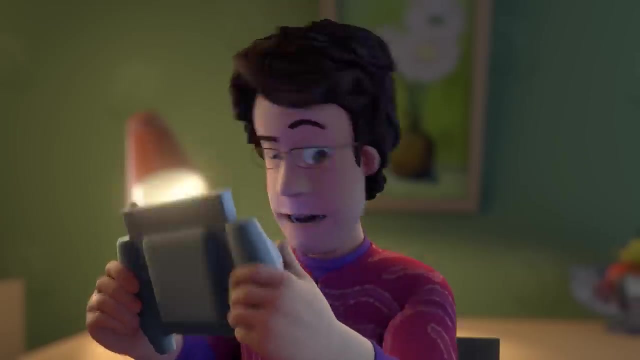 There are also robots that can understand what people are saying, And robots that can talk and even make jokes, just like people. I've got it. Now let's turn you around. Let's see what you can do to help us, Uh. 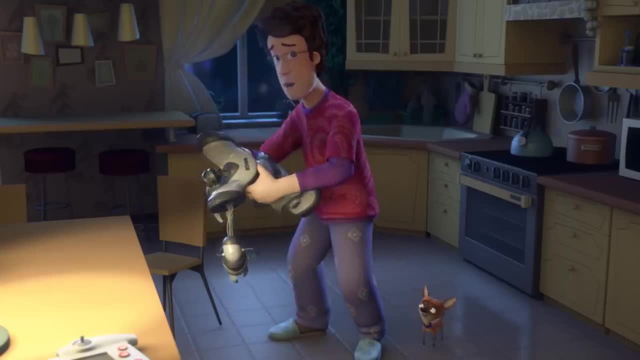 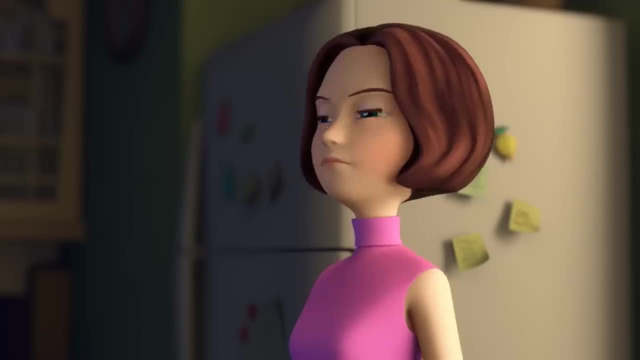 What was that? Uh, look, you know, He destroyed him. Nolik, stop, You were playing with that, right? You think Tom will notice. Oh, I know what you're doing all night. I'm off to bed. 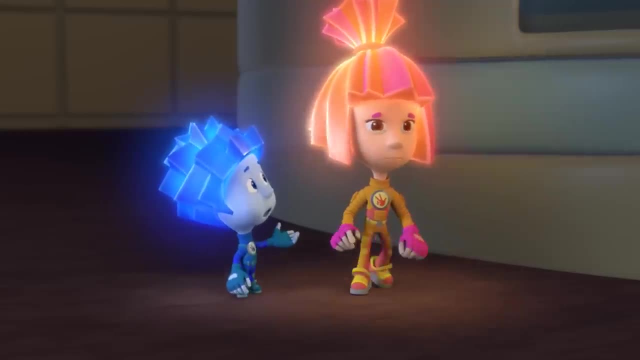 I'll get him to work. I'll stay up until I do. Simka, let's try, and No, we're gonna need some help. Nolik, stop, Simka, let's try, and No, we're gonna need some help. 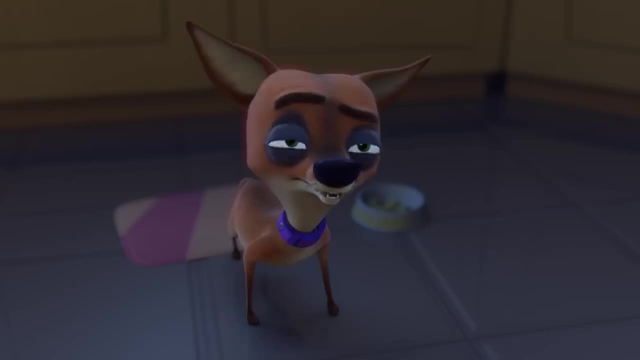 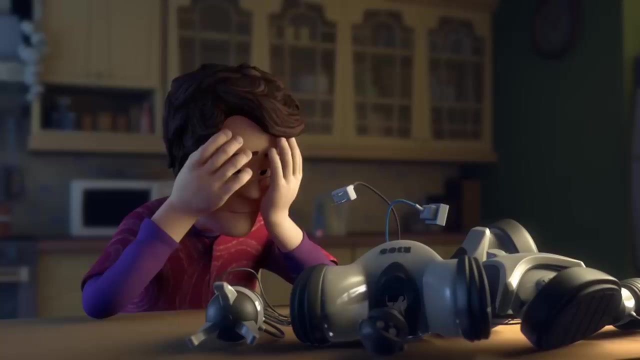 Simka, let's try. and No, we're gonna need some help. Simka, let's try. and When your TV has broken, When your cell phone has croaked, Your laptop's barely working, The kettle's had a stroke, Don't ask us where we're going. 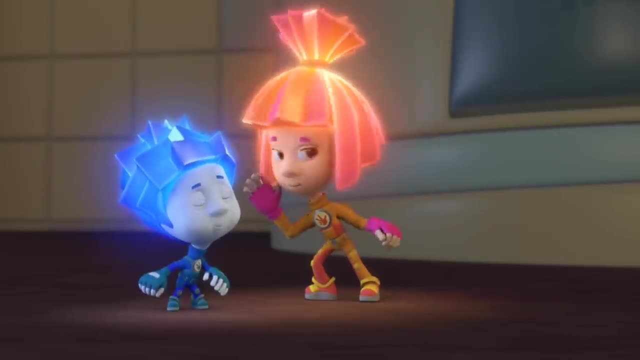 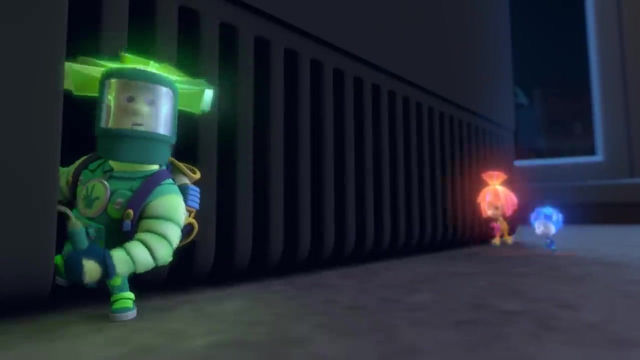 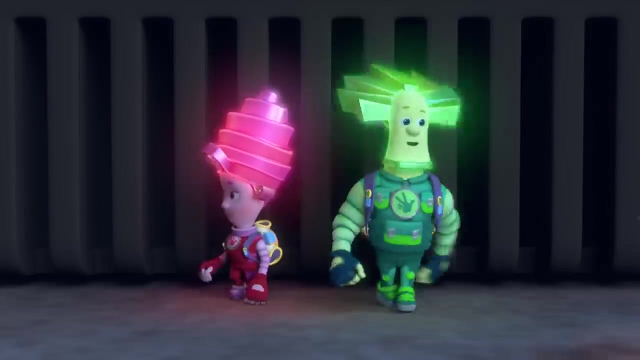 For it's known far and wide That any kind of problem Is clearer from inside. One, two, three Tideesh Inside. we'll be Tideesh To fix what's wrong. Tideesh Till it runs strong In gadgets and devices. Our work will never end. 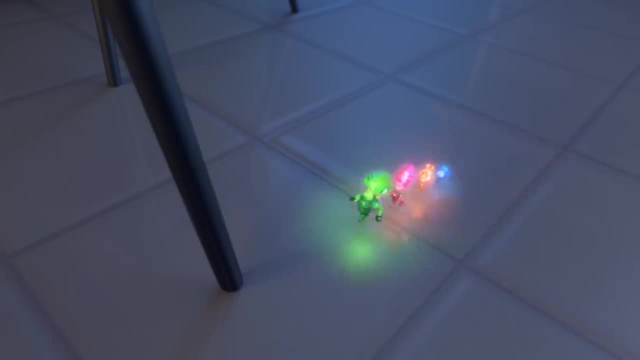 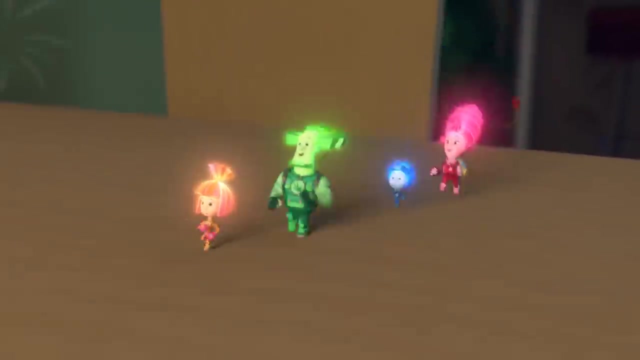 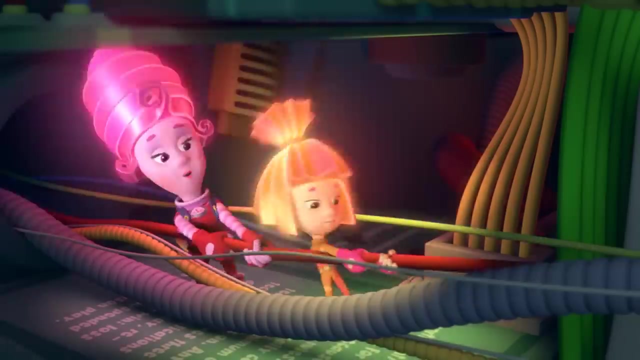 Applying. Our devices are fickle. They need a loyal friend. At morning, noon and midnight Of every single day When there is an emergency, You know we're on our way. One, two, three. Inside we'll be All day and night. We fix things right. One, two, three. 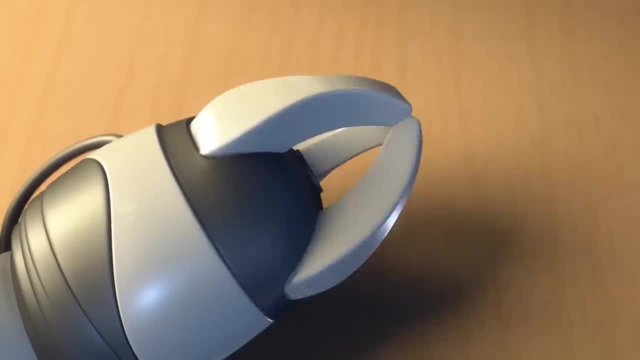 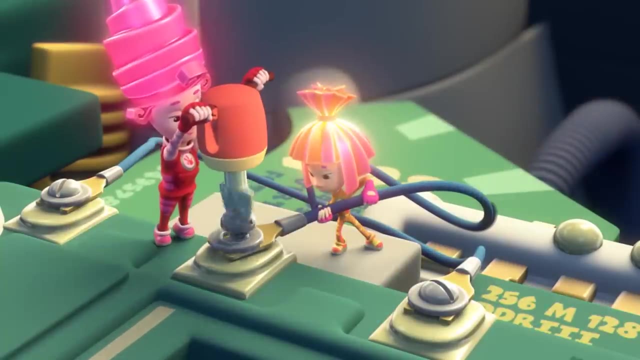 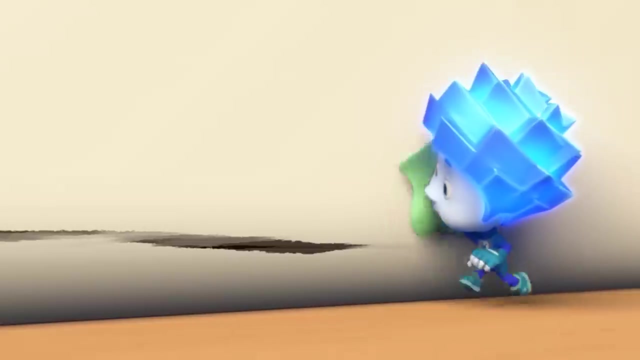 Inside we'll be All day and night. We fix things right. We live to keep On working, And work for us is fun. So we'll just keep on working, Cause our work's never done. And deep inside of gadgets- If you look when it's dark, You might just see us. 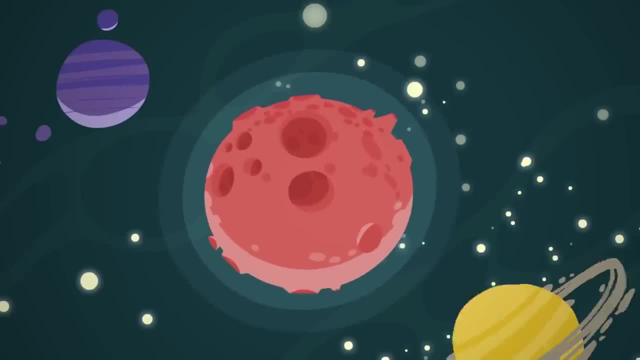 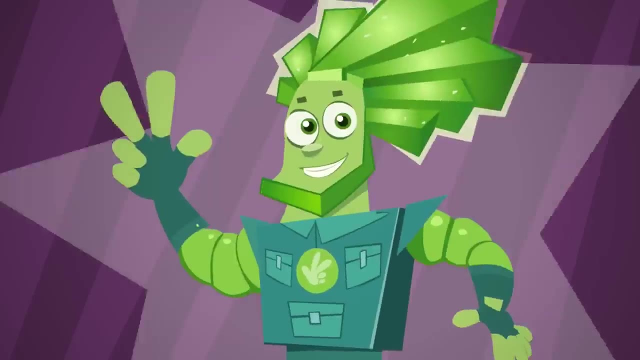 Ranging around like multicolored sparks. One, two, three Tideesh Inside. we'll be Tideesh To fix what's wrong. Tideesh Till it runs strong. One, two, three Tideesh Inside. we'll be Tideesh All day and night. 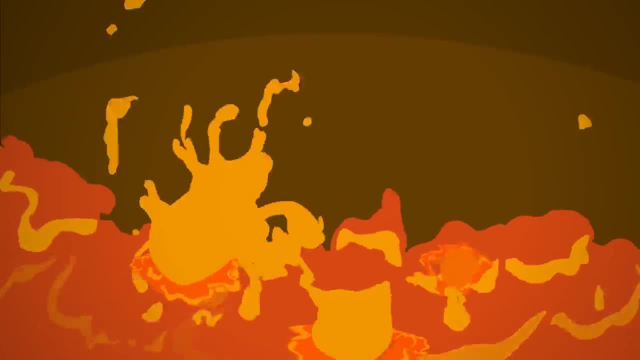 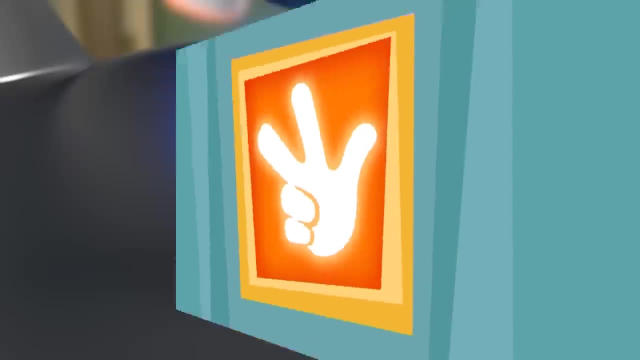 Tideesh, We fix things right. One, two, three Tideesh Inside. we'll be Tideesh To fix what's wrong. Tideesh Till it runs strong. One, two, three Tideesh Inside. we'll be Tideesh All day and night. 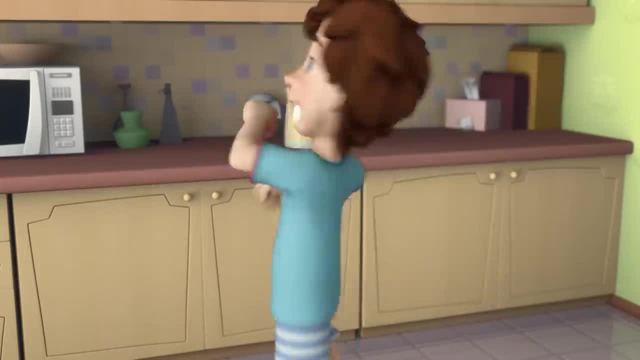 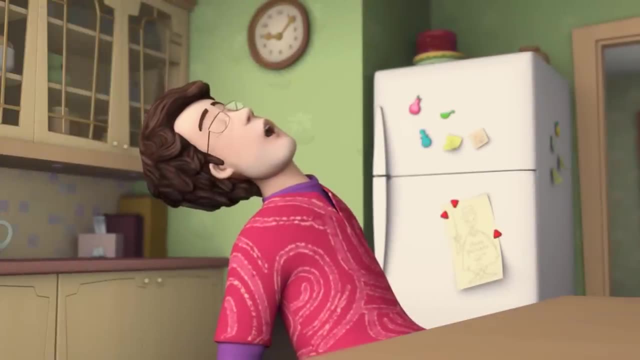 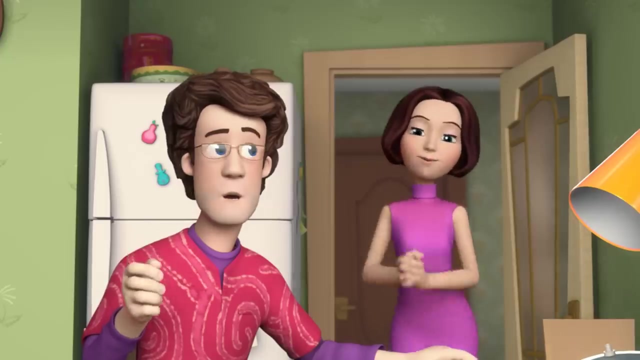 Tideesh, We fix things right. Wow, you got it. We need to hide A Robotozoid R300,. I can't believe it, Wow. Hmm. Well, happy birthday to you, Tom Thomas. I'm sorry, Tom Thomas. 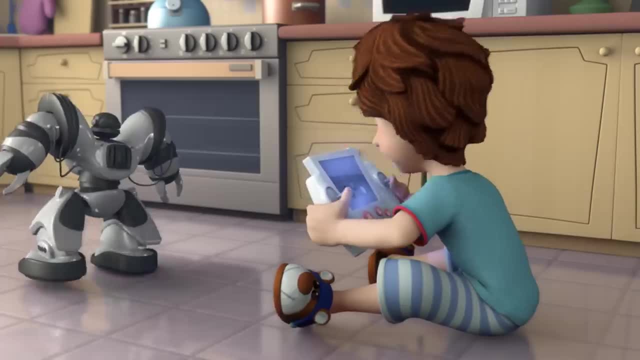 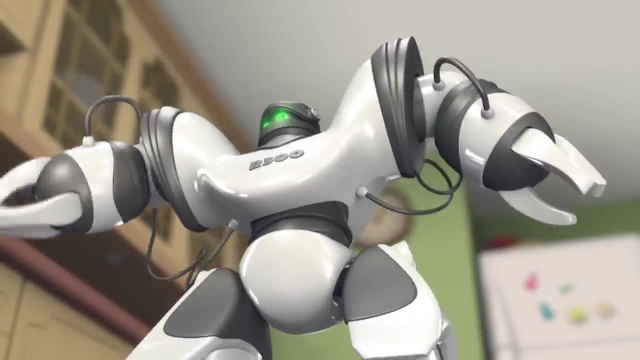 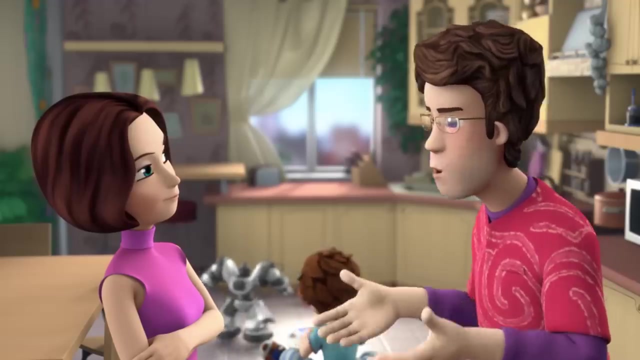 Last night your robot- you know, I broke it, Dad- it works perfectly, Don't you see? I'm so proud of you. You fixed it. Shh, I couldn't fix it at all. I tried everything. Oh, you want to tell me that the robot fixed itself? 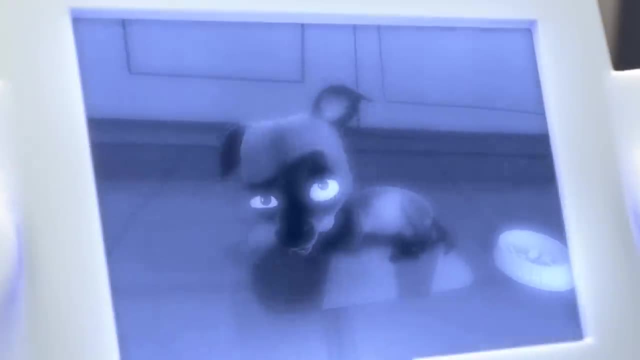 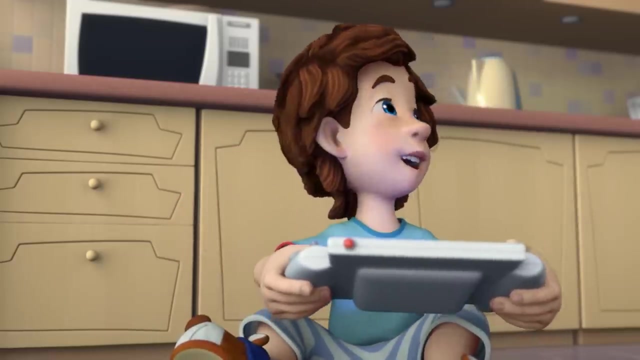 What a joker, Mom Dad, thanks so much. Bye, Steve, Byequit. See ya, You shoot this robot. I can't do it. No, not the robot, I can't Fall away. Mom Dad, Thanks so much. 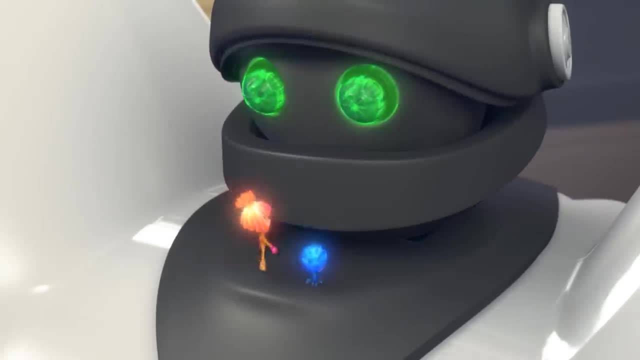 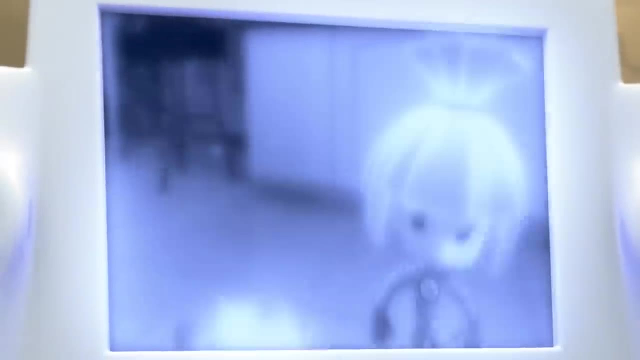 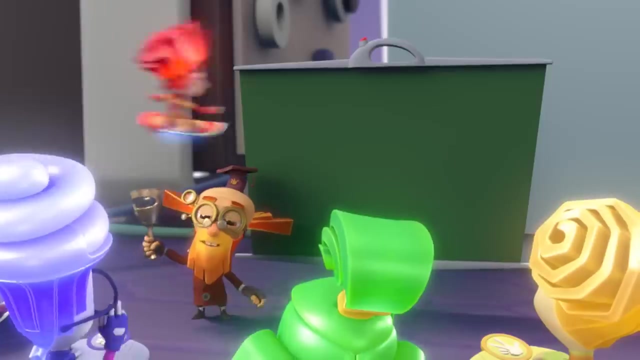 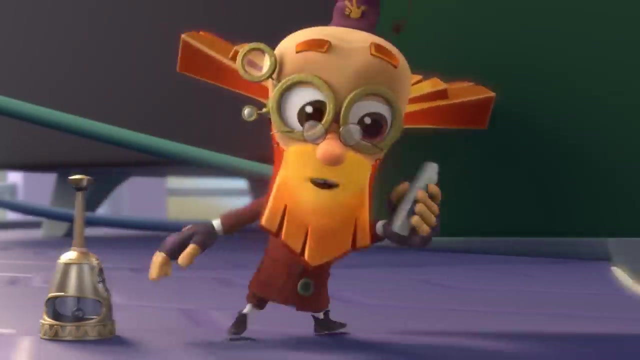 I love it. You, son of the population man, How about thanking us? I should've known it was you who fixed the robot. Happy birthday, Happy birthday, Quiet down. Get ready for For your lesson. be quiet, quiet down, please. Oh, it's so hot here. in today's class We'll learn about 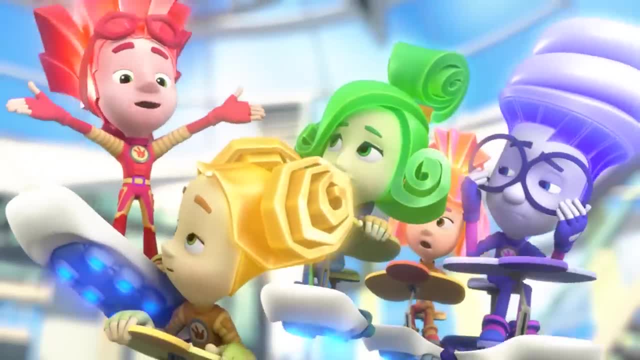 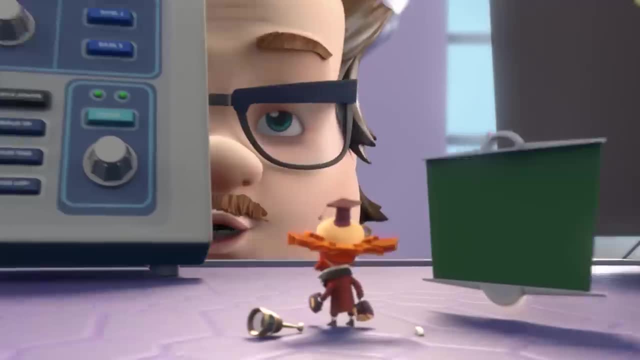 It must have been an earthquake. Yeah, it was an earthquake. Hooray, Sorry there, professor. Oh, I have to find an outlet so I can plug in this fan. Oh, It feels terribly hot. It sure does. Well, keep looking, you'll find one. 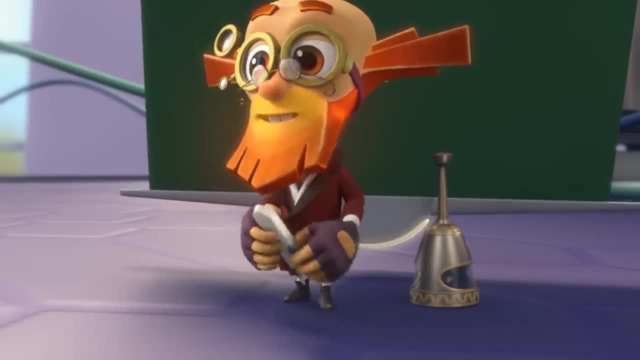 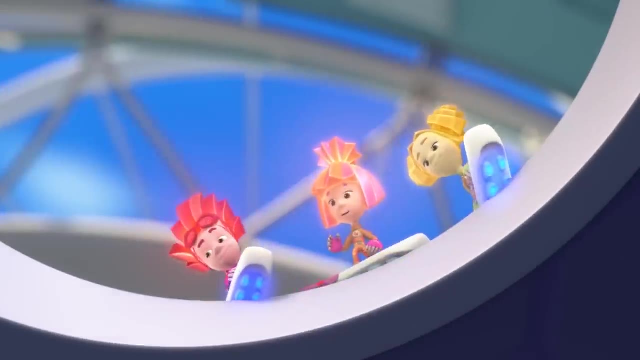 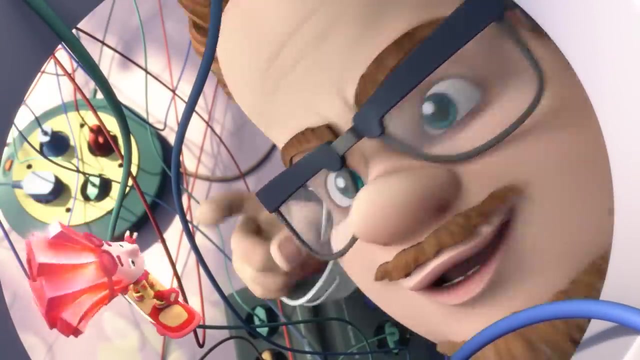 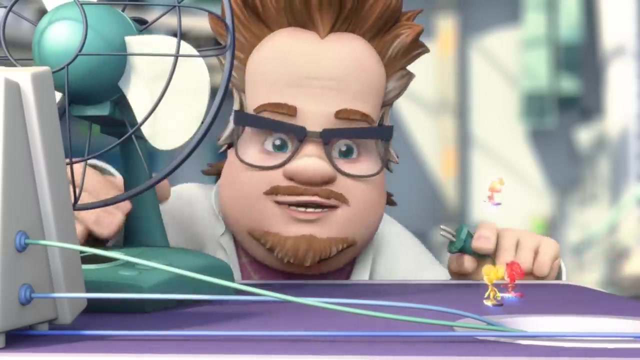 Oh No, it's impossible. in this whole laboratory there isn't one free outlet. look at this: Just pull out one of these wires and then you'll have a free outlet. I can't. I Fear I could pull out a plug for something important. Ah, bolt himself would get all tangled up in these wires. 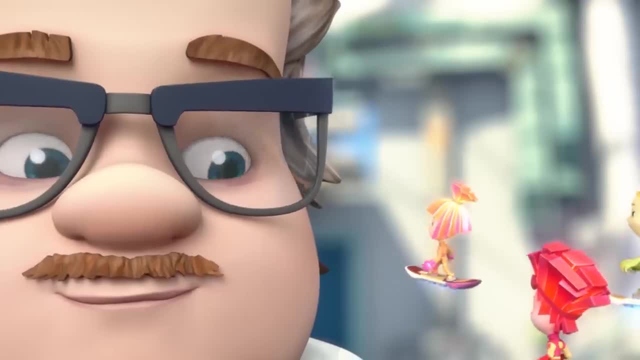 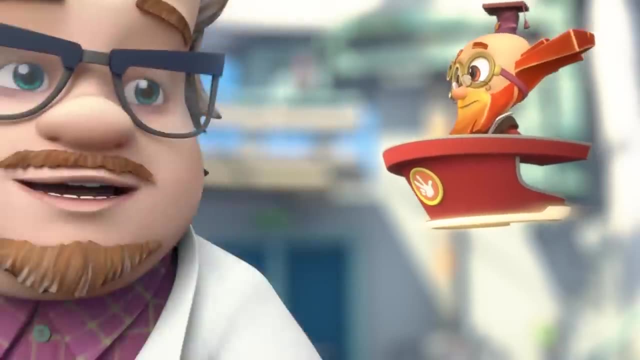 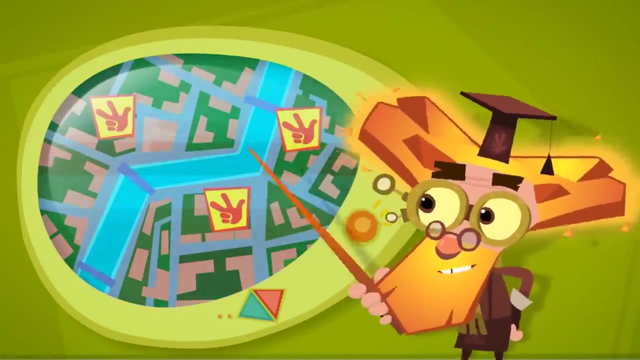 Don't worry about it, professor, you genius, We'll find a free outlet for you. That's right, My colleague. a cup of tea will do you good, So just go relax. Thank you, my colleague, and as always, I'm eternally grateful. Fixies have opened schools for their children in all sorts of different places like factories, stores and warehouses. 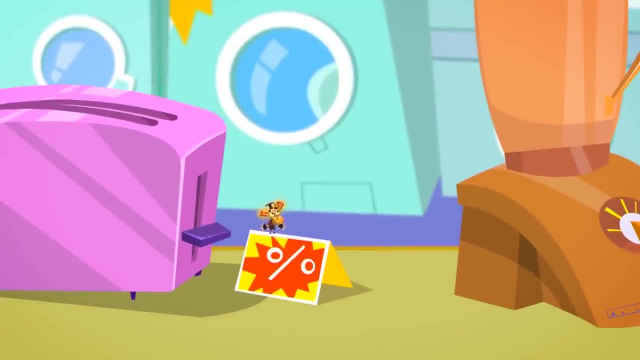 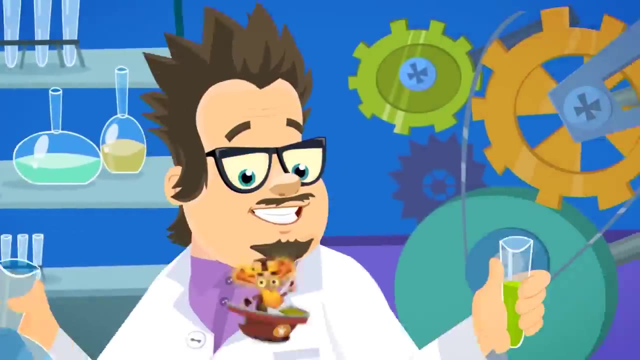 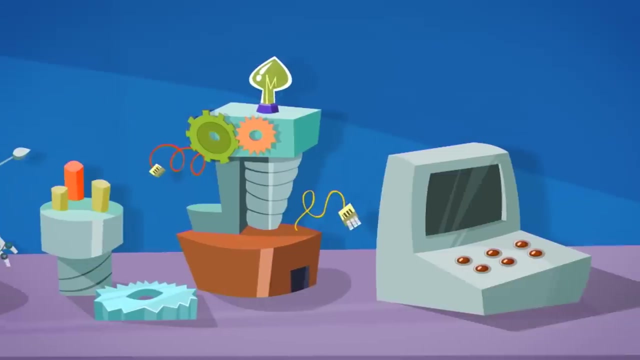 Anywhere where there's lots of machines and appliances and places to hide from humans, and this is where we hold our school, right here inside the laboratory of professor you genius. It's a fantastic place for me to hold class. every day, new devices, materials, toys and even food are brought here for 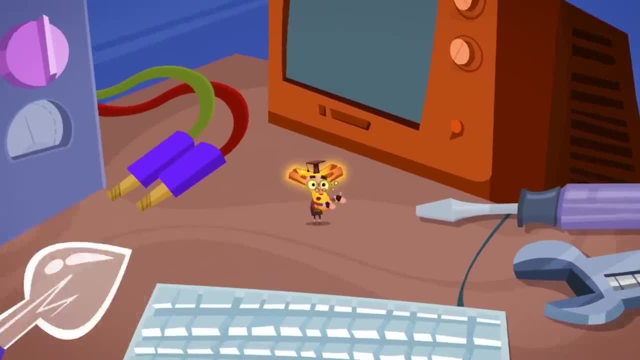 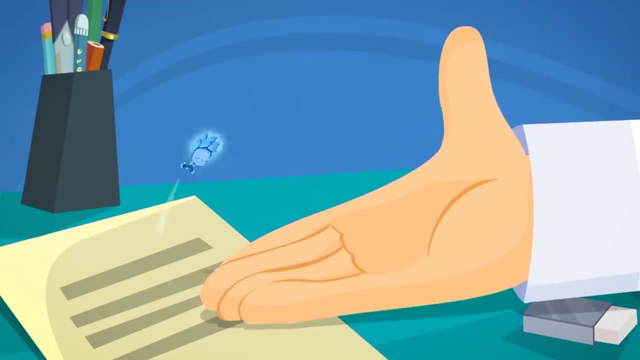 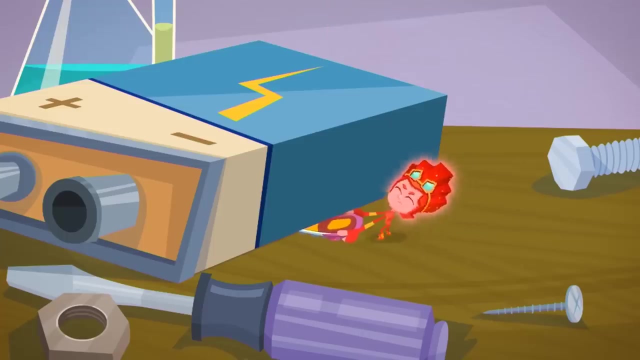 Examination, and there are lots of scientific devices and tools to study here as well. But, most importantly, we never need to hide from the head of the laboratory Because my colleague, professor you genius is someone I'm proud to call a friend. He loves fixies, helps us anytime we need, and we'll never let our secret out. 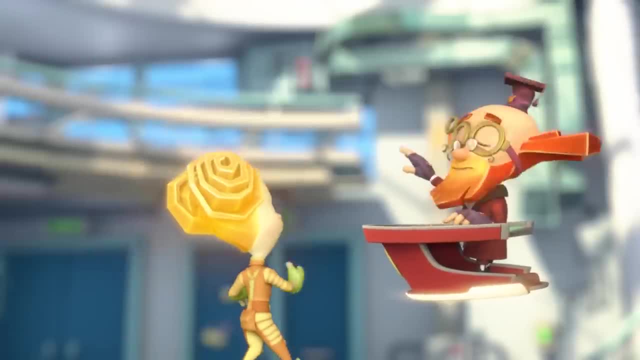 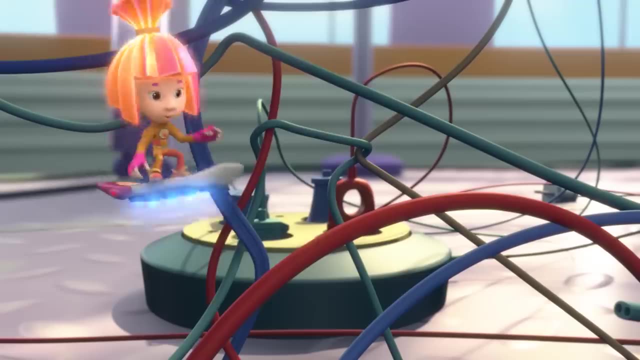 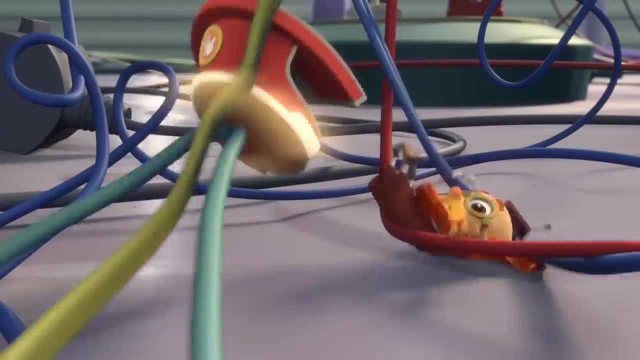 He loves fixies, helps us anytime we need and we'll never let our secret out. What should we do first? we have to start out with pulling apart these wires. that'll take a second Over here. Over here. No like, come on, let's do this Over here. 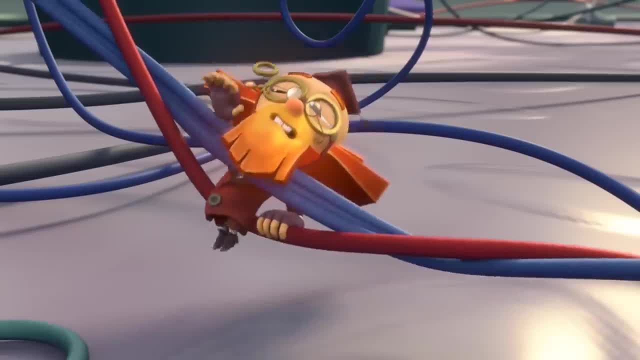 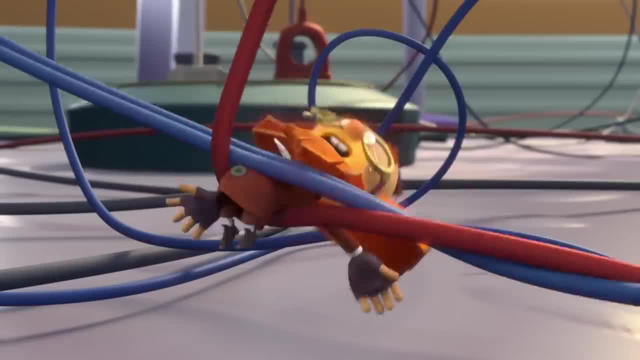 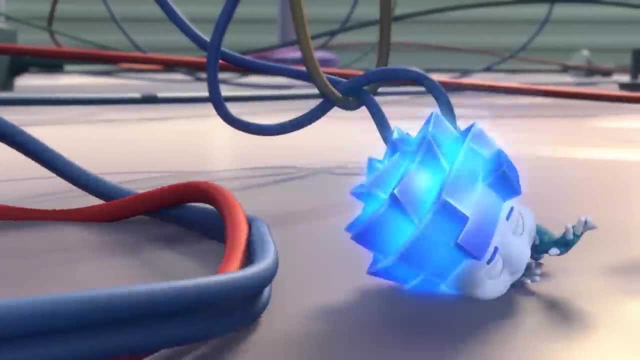 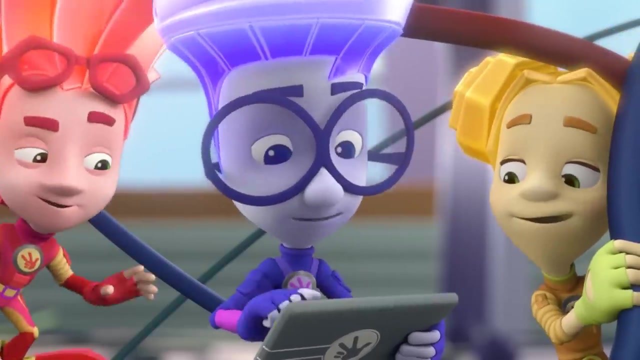 We need to pull out this one. We need to pull out this one. We need to pull out this one. Stop this nonsense, will ya? Thank you, Digit Tideesh. Well, the way I see it, in order to get the knot out. that's over here. 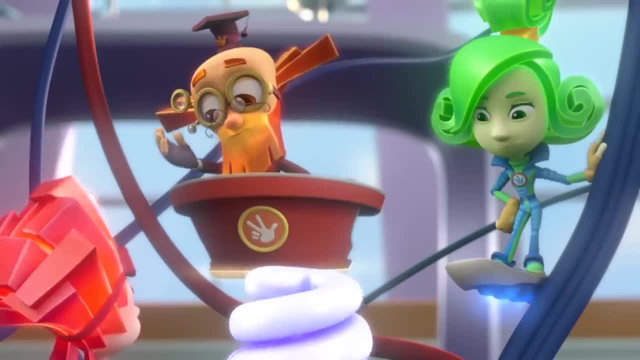 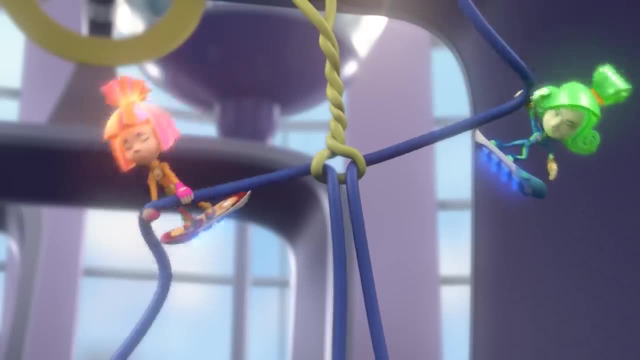 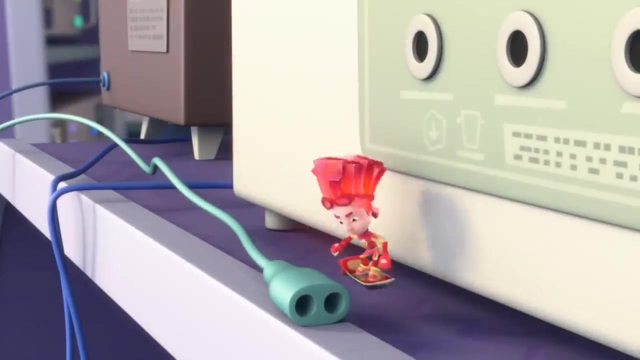 We need to expand the loop that's over there and then push that wire through it And then do it again from the other end. That's it, Very good girls. Hey, Now pull it hard. Perfect. Hey, check it out. The screen wire up here isn't plugged into anything. 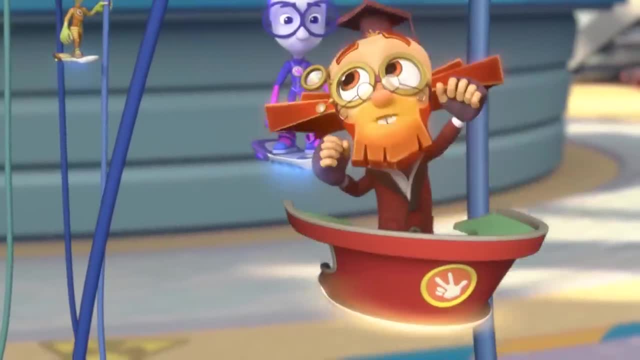 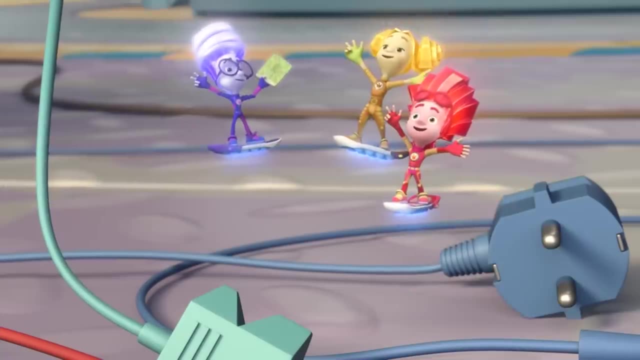 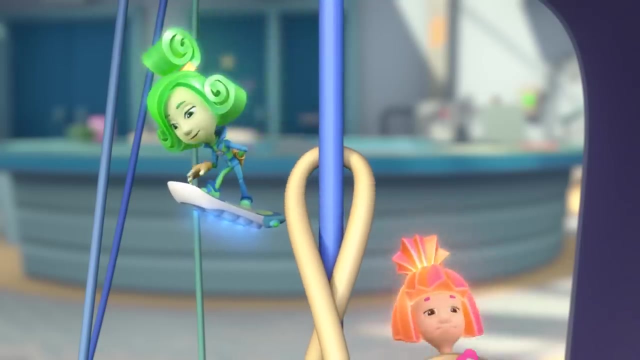 Then no one's using it, So that means we should go and pull it out from the outlet. Got it, Tideesh Verda? here's another wire that isn't plugged in. I found another wire no one's using, And I mean Simka and I found it together. 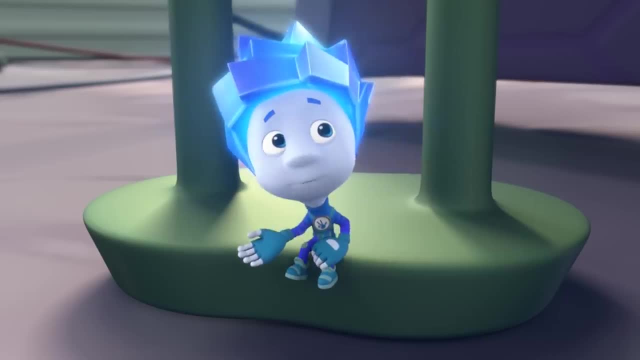 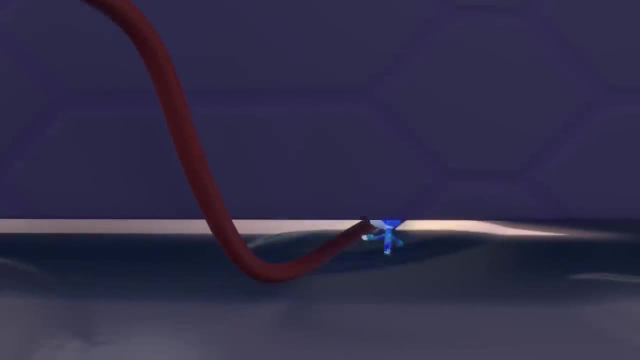 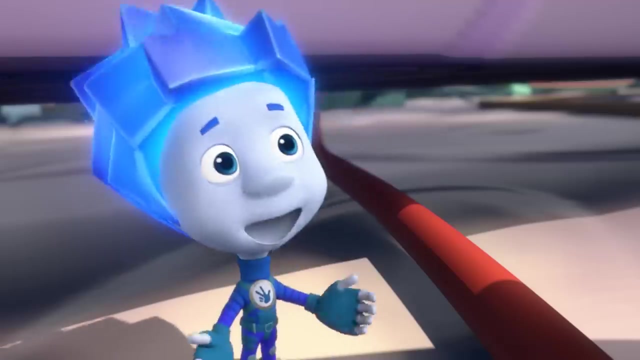 Nolik, why are you so upset? Because you guys are doing all the work. How about this wire? Nobody's checked it yet, Really, Oh wow, What Did you find? some treasure, Nolik. Uh-huh. There are six free outlets under here. 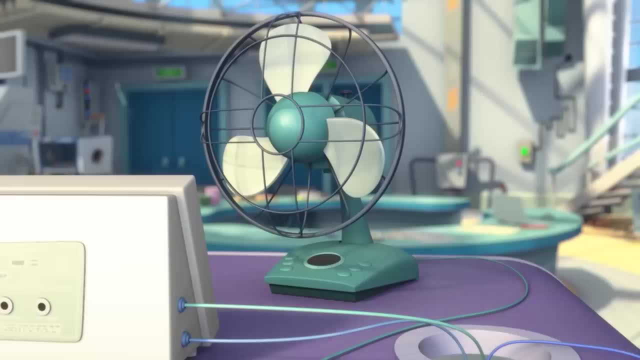 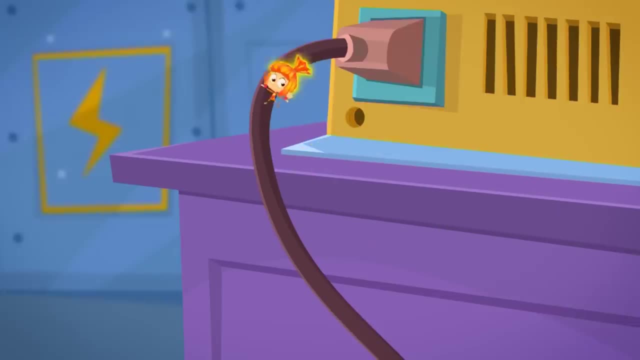 Great. Now Professor Eugenius can pull out and plug in his fan and his kettle and even his soldering iron. To get electricity to a device that doesn't use batteries, you need to plug a pair of wires into an outlet. 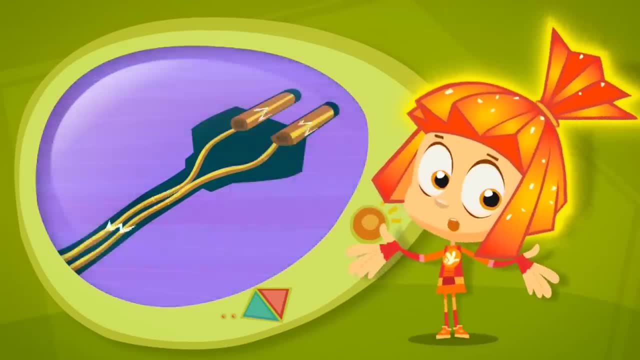 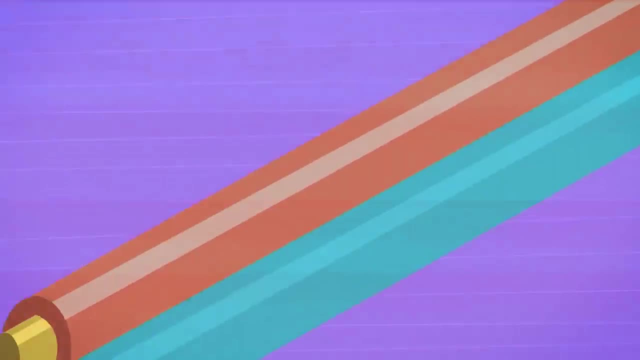 But it's important not to let the wires touch one another, or the electricity can burn them out. That's why wires are covered in plastic or rubber, so the electricity won't pass from one wire to the other Or to us when we touch them. 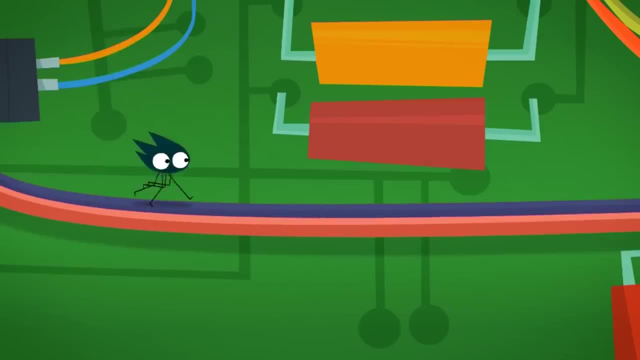 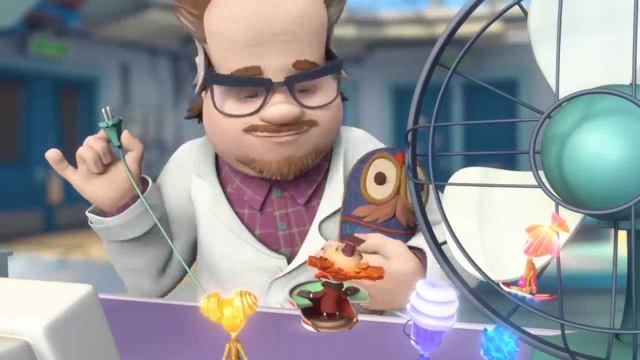 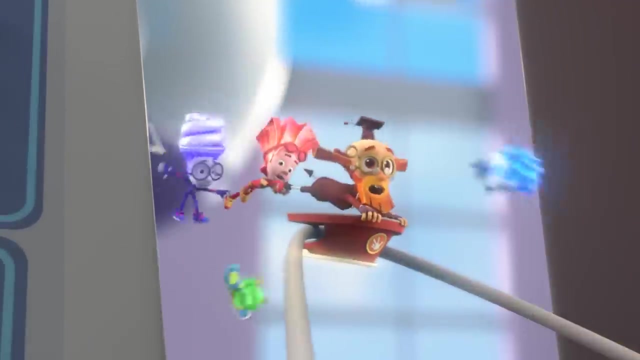 So always be very careful with wires And never, ever touch a bare wire. You could get killed by the electric shock. Oh, what would I do without my wonderful friends? Thank you, Ah, sorry, I just I didn't. I wanted to. 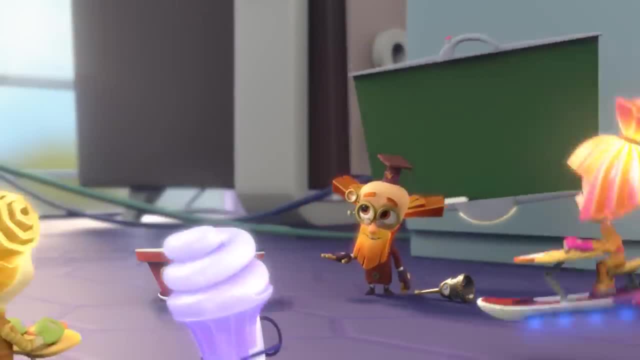 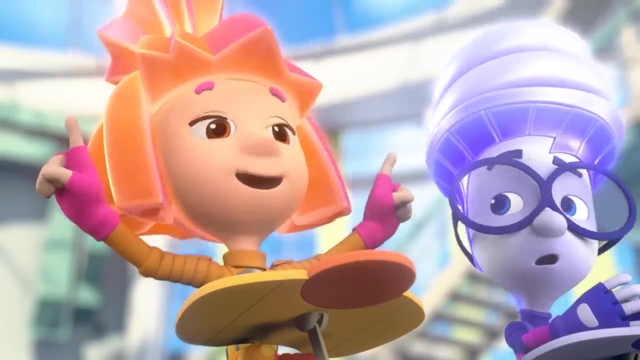 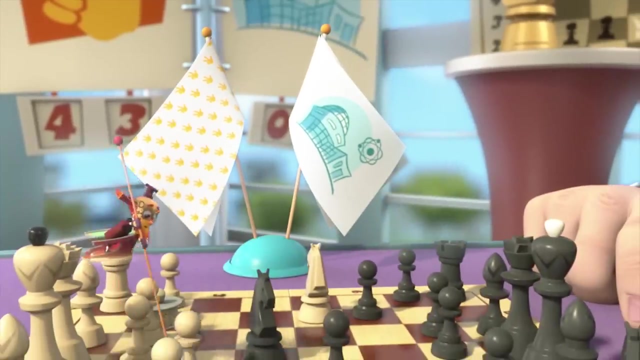 I should go Go ahead, That's a great idea, And we'll start our class. Uh, what were we talking about? All about wires. Well, it looks like our class is over Time to go play. How about that? 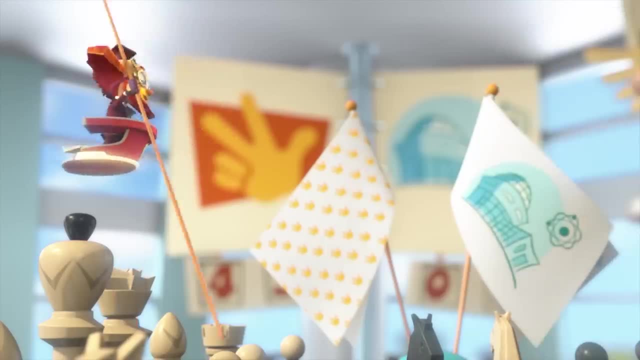 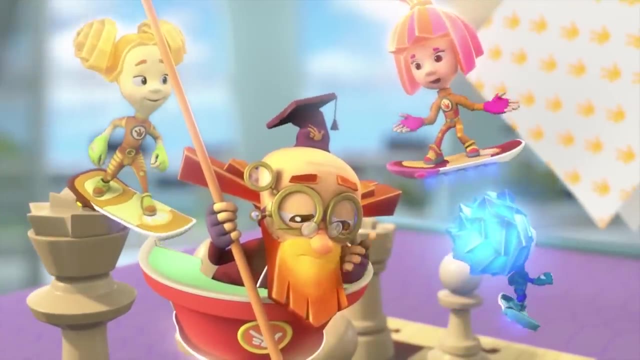 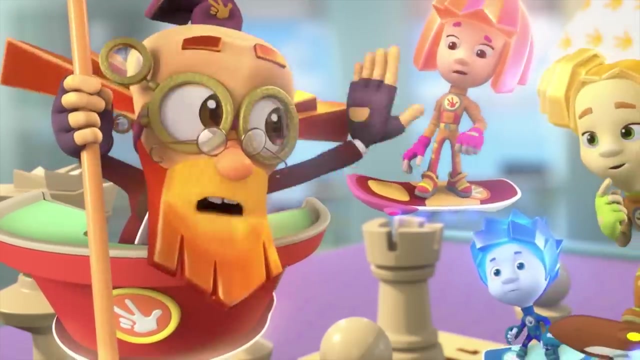 Then I'll play my pawn, And I'll play my pawn. Grandpas, we need our spool and it's missing. Oh, congratulations, Professor. have you seen it anywhere? The spool? I haven't seen it. We're playing chess. 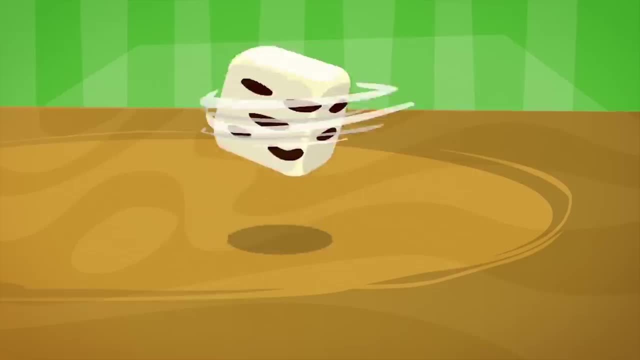 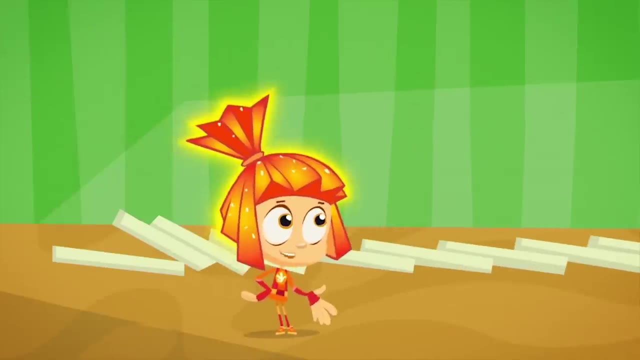 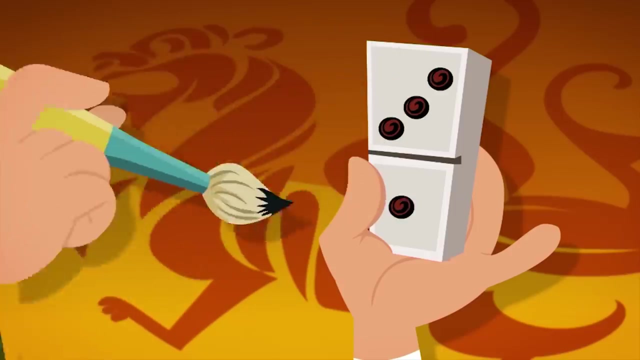 Can't you see? Do you like board games, Like Dominoes, for instance? Just about everybody has played it. But do you know where it came from? Dominoes was invented by the ancient Chinese. They made tiles and decorated them with dots, like on a pair of dice. 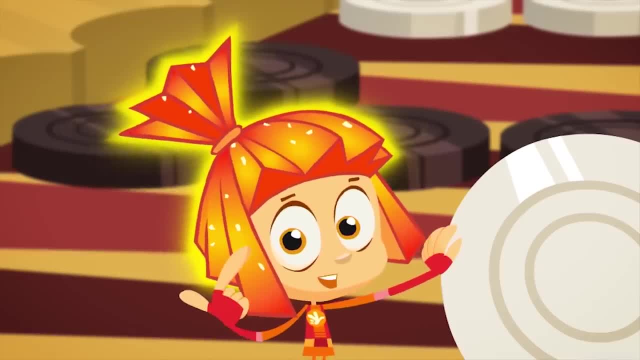 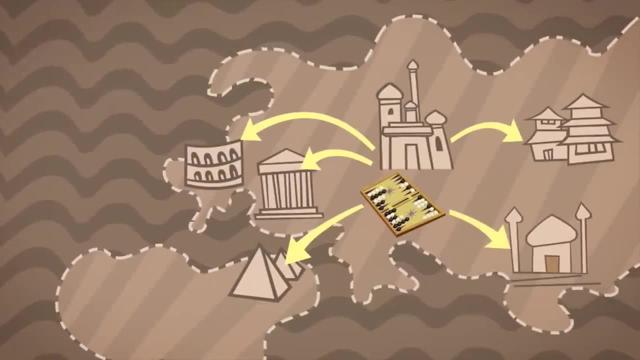 And this is a game that looks a lot like checkers, but it's a lot more challenging. It's called backgammon. Backgammon originated in Persia and from there it spread all over the world. But the most challenging game of them all is the game of chess. 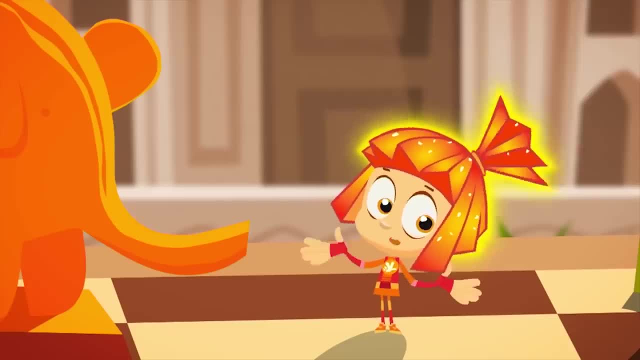 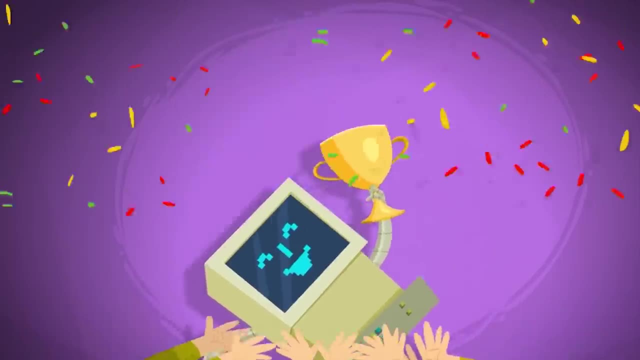 Chess was invented in India, and today the game of chess is loved in every country. It's played by adults, by children and even by computers. Chess is a real sport, But the most important thing for playing chess is not the power in your arms, but the power in your brain. 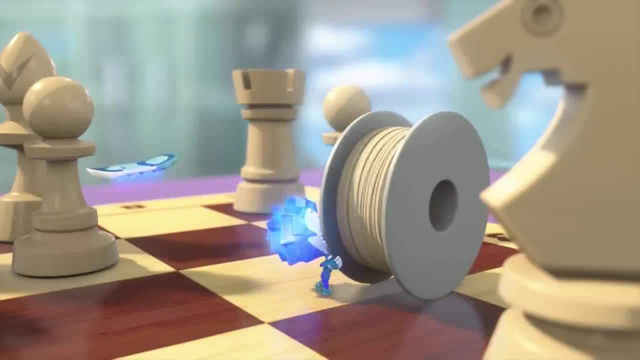 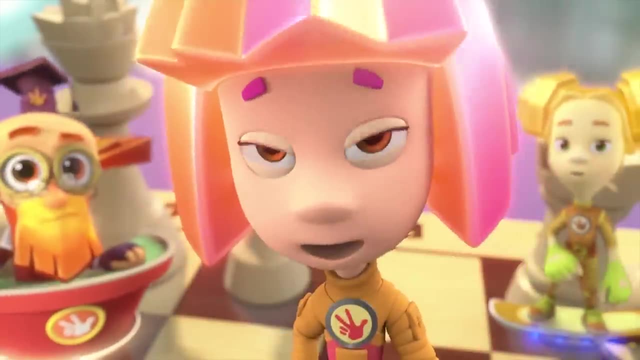 Hey, look, I found it. Yeah, Hey, Hey, What's going on? That's our spool. Please let us take it back. There's something we have to do with it, But we're using it, Can't you wait? 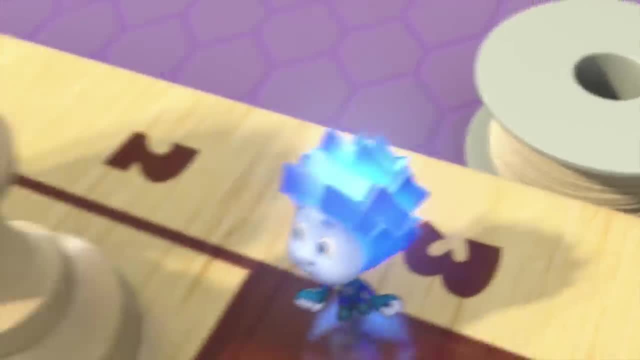 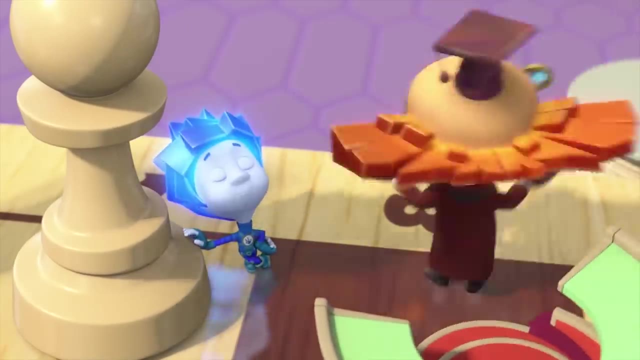 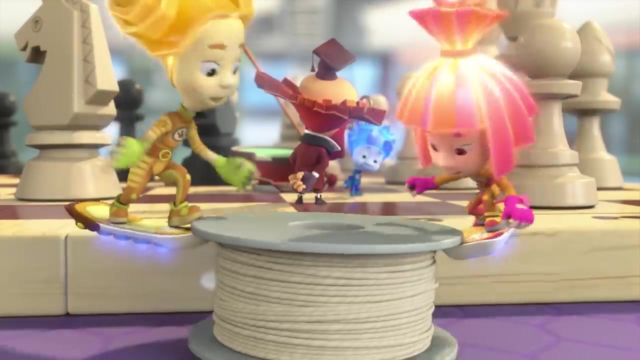 It's a replacement for the missing pawn. Oh, Oh, Nolik can work for a while as the pawn's replacement. Yeah, I can do it. Alright, You can take it And you stand right over here. One, two, three up we go. 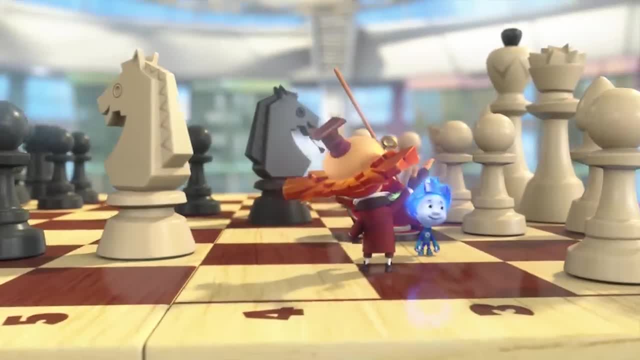 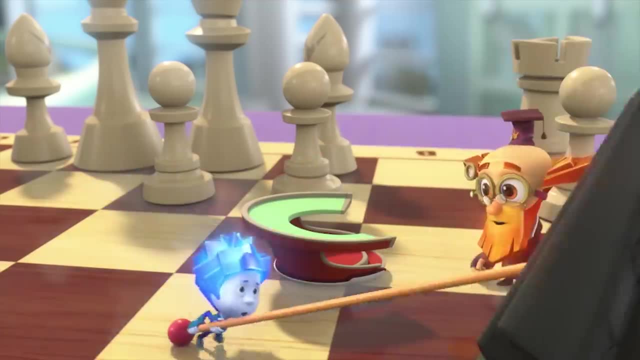 Class. So how do we play? You're going to play for the whites And now I'm going to capture your knight And we We're going to knock over yours. Take that. Whoa, whoa, whoa, young man. 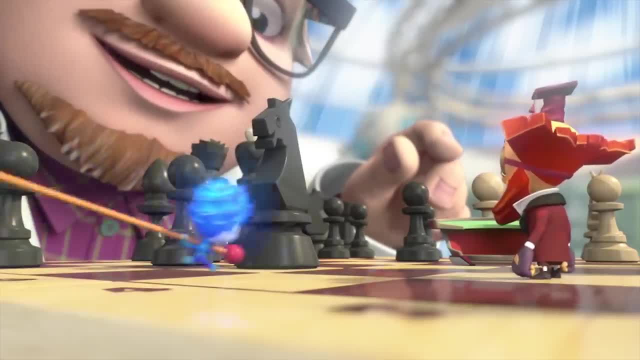 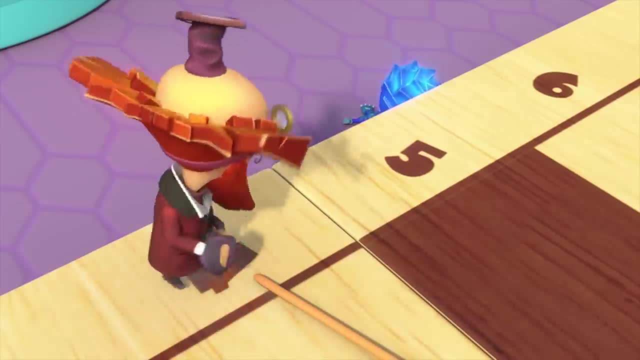 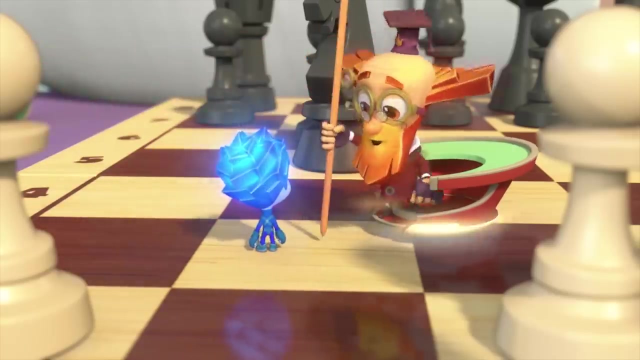 Slow down. It goes back here, Nolik. get back to your square. What for Pawns don't move like that? And how do they move? Only one square per move And only forward. Of all of the pieces, the little pawn is the weakest. 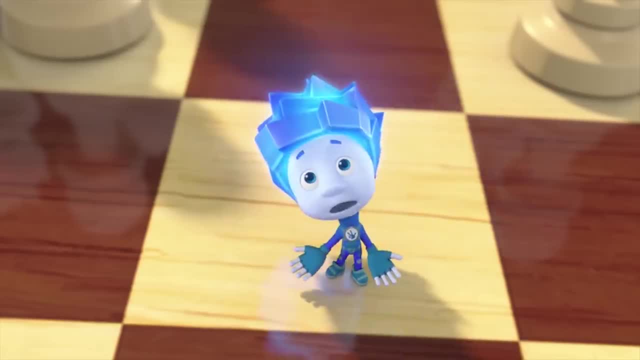 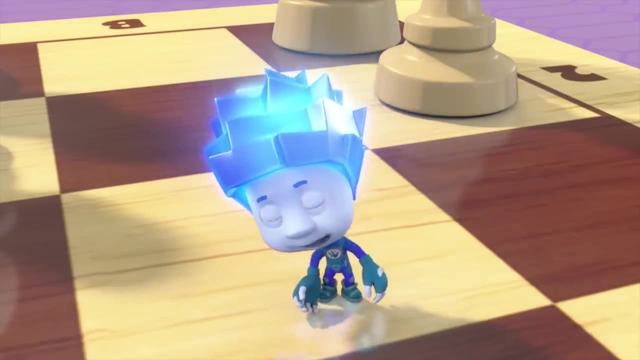 What a mess. So which one's strongest? huh, This, It's the queen. She's the most dangerous threat to the other king. Aw, how come I couldn't be queen, Then that black king would have to deal with me. 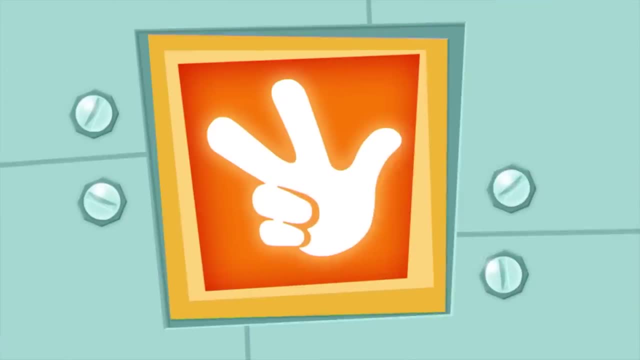 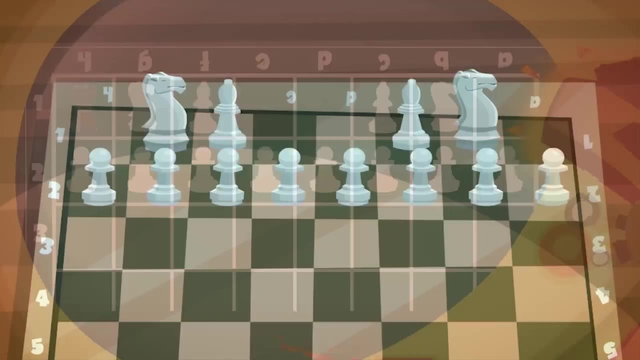 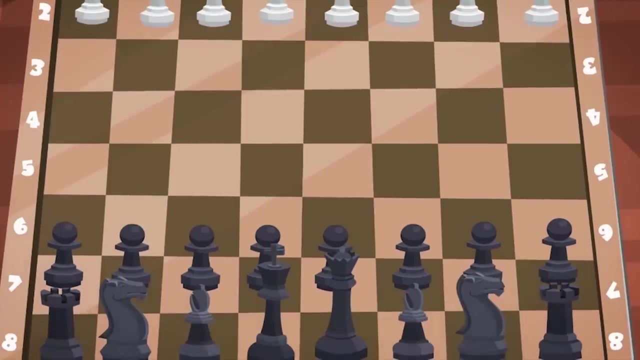 Oh yes, In chess, each player has a black or white army with eight pawns, two knights, two bishops, two castles and a queen. All of them, All of them work together for their king, trying to protect him while attacking the enemy's king. 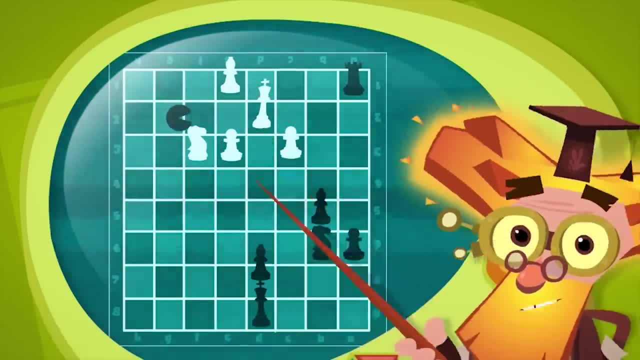 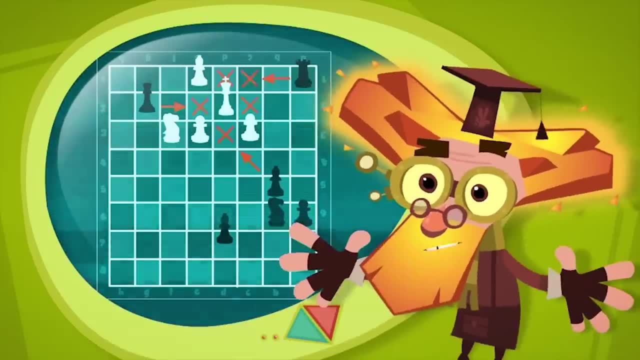 If the king finds himself in a position where he can be captured, the attacking player says check, And if the king finds himself with nowhere to run from the attack, it's called checkmate. Whoever checkmates the other player's king first is the winner. 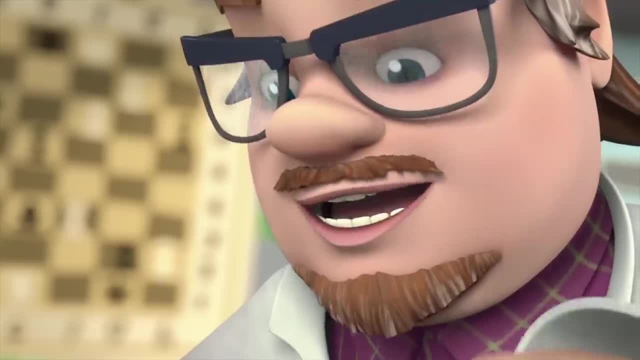 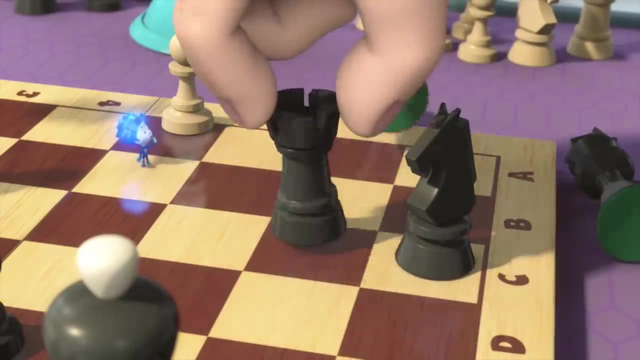 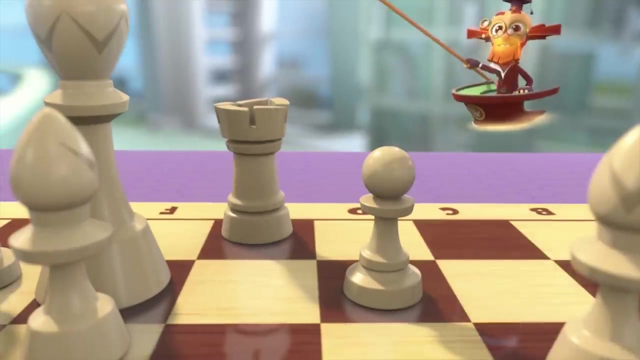 Hmm, I'll move my queen, Yeah, And me my queen. Then I'll just capture your queen. Aha, Really, Then I'll just capture yours. Grandpus, should I go now? Not yet. So do you feel like surrendering? 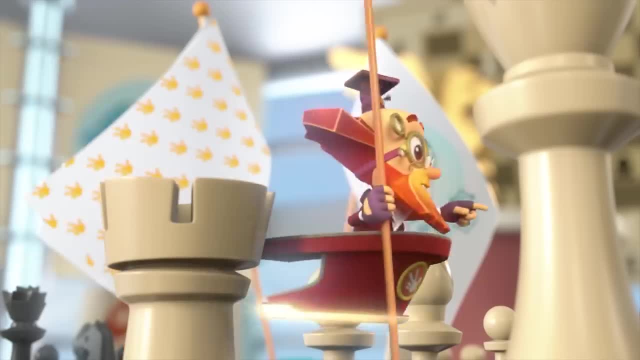 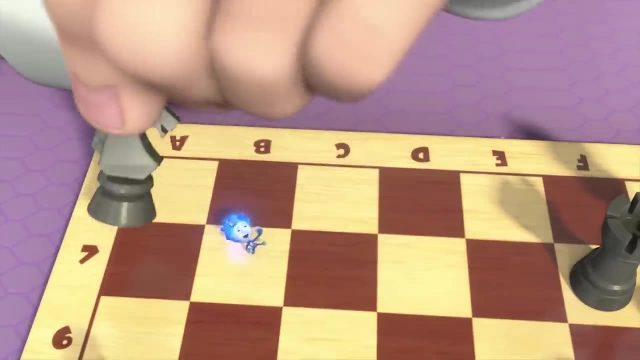 Ha, you're kidding, do you? Nolik forward, Hooray, We'll step aside Forward, Aha. Next I'll go and capture the knight. He got away All right, pawn and once more, go forward. 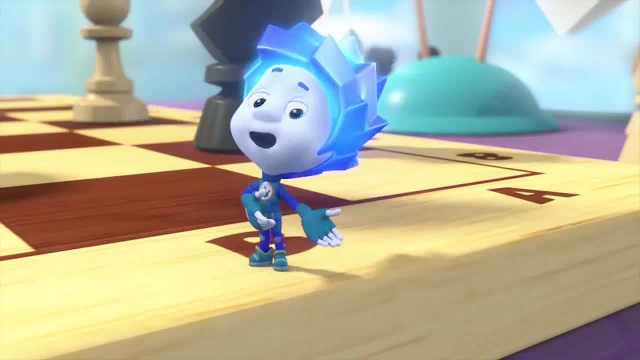 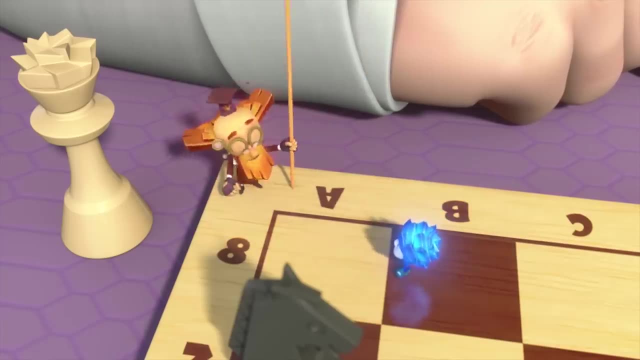 Gra-grandpus, Where do I go now? Don't you see the edge? Don't go anywhere. Now you're the queen. What? The rules of chess say that if a pawn makes it all the way to the other side, he can become anything that was captured earlier. 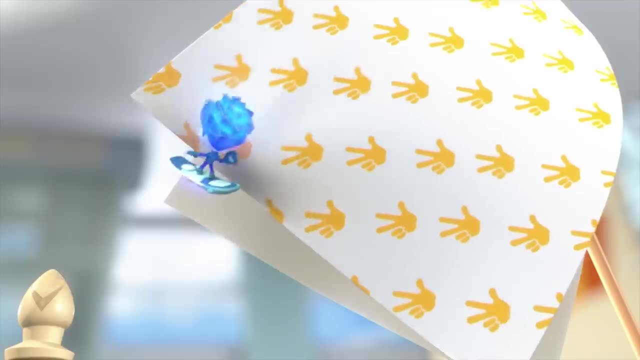 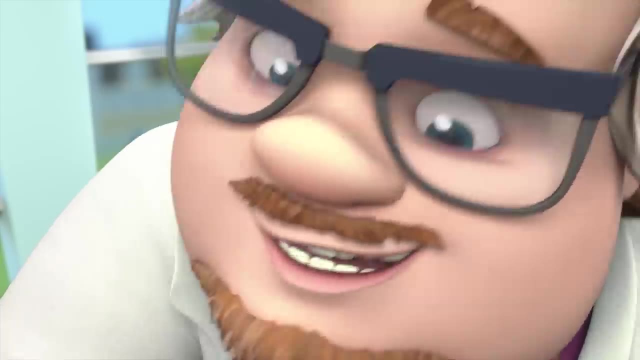 Hooray. Then I'll be the queen And I'll be the strongest piece in the whole game. Hey queen, Get back here. In case you don't know, this isn't over yet. We capture the pawn with the queen. 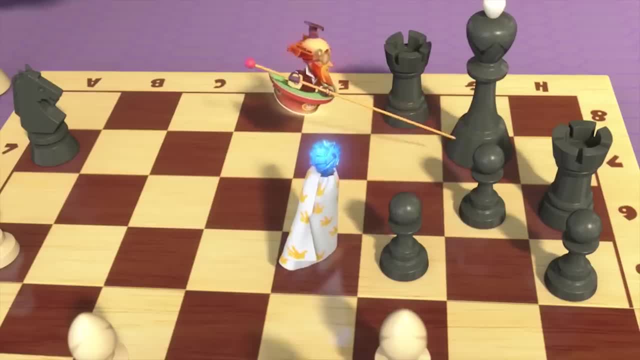 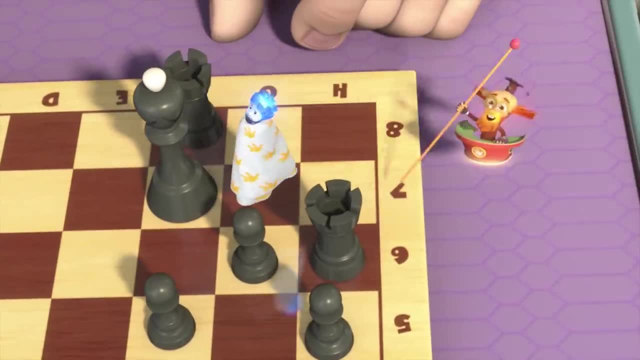 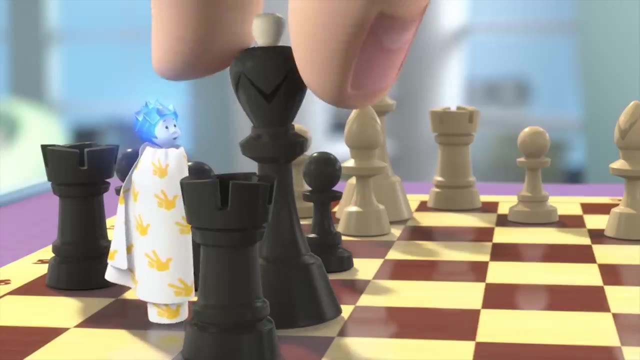 Queen, this is your new place, Check, Check, Huh, yeah, Heh, Now come to here, Checkmate my colleague. Of course it is. It is mate. Yeah, I lost Hooray. Tideesh, tideesh, tideesh. 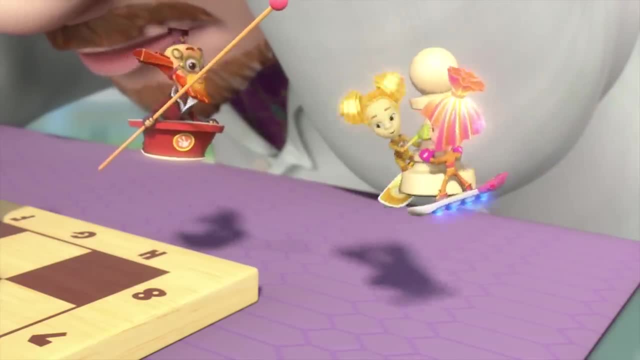 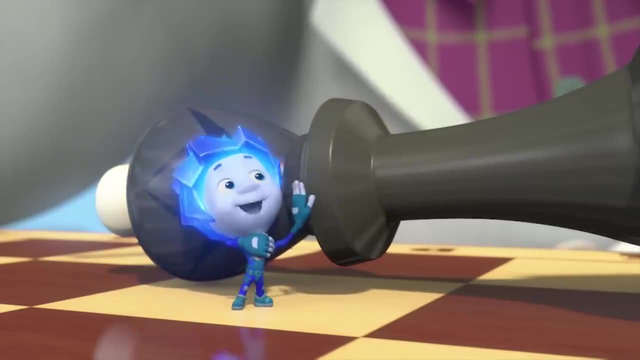 Professor, we found the missing pawn for you, So that means Nolik can leave with us. I'm not going anywhere with you. Chess is the greatest game you'll ever play in your life. Oh, you should have seen how I put Professor Eugenius into checkmate. 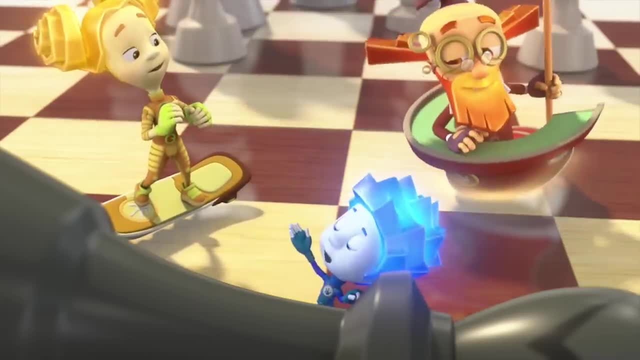 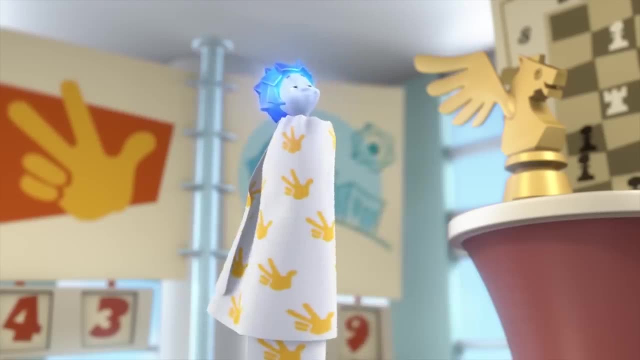 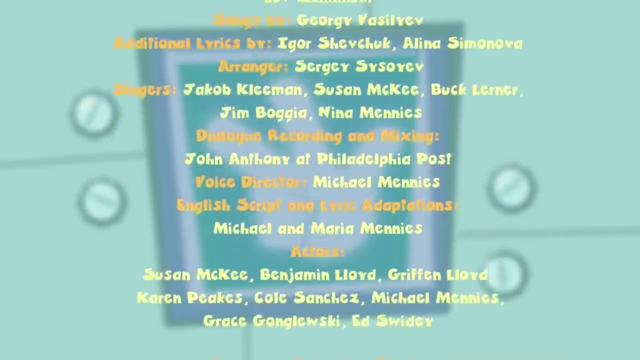 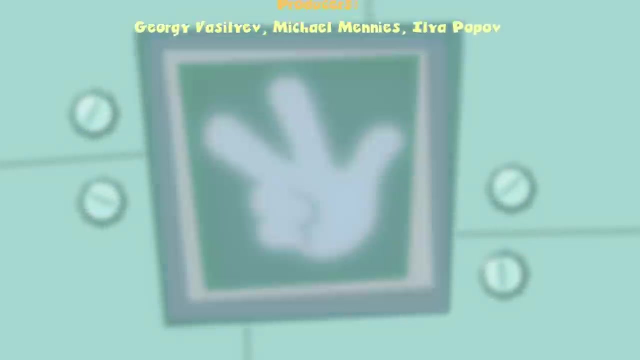 Really Well. Grandpoo's helped me a little. Actually, it was Grandpoo's telling me where to move, But I'm the queen now. Please don't let their secret out. Subtitles by SteamTeamExtra.